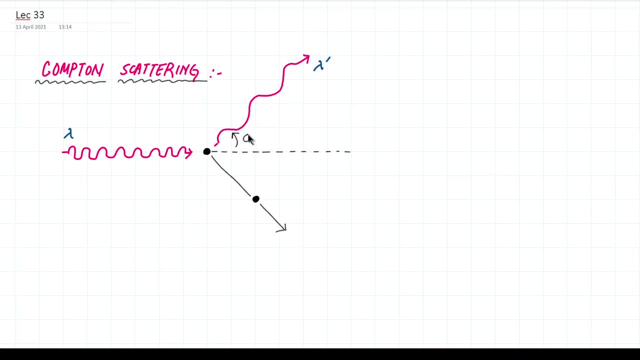 So let's suppose theta is considered. Everything else is usual, The energy momentum, etc. etc. etc. Now I don't want to solve this problem using the obvious approach, which is momentum along x axis, y axis, Apply conservation. Do some mathematical calculations No? 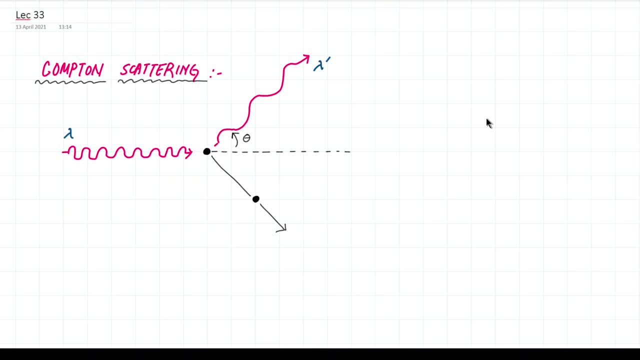 I want to use the concept of four vectors and see how it is different. Can it be done? If it can be done, what to do? You are familiar with it. We defined four vectors, or the energy-momentum vector we defined. We defined the energy-momentum vector, which was p nu. 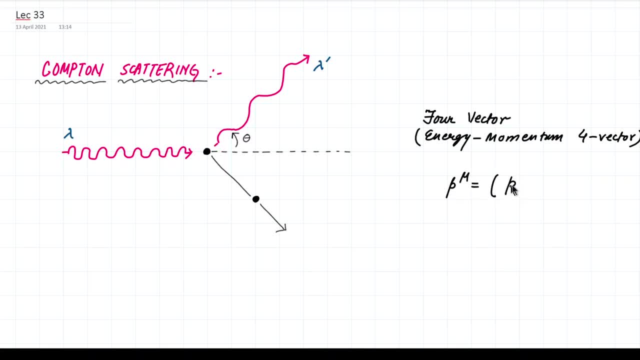 In p nu you had four components: p 0,, p 1,, p 2 and p 3.. So the zero component is nothing but the time component, And I showed that the time component is equal to total energy upon c. 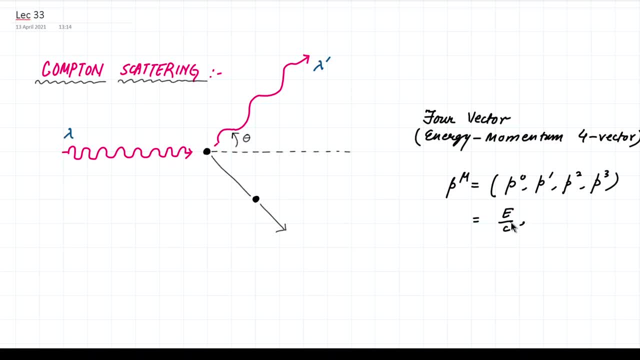 And this is true for photons as well as particles and everything else. And the rest are the components along x, y and z axis, The ordinary relativistic momentum components, And I also showed that That one concept we will need to use, that the inner product, or scalar product, or the norm of the four-momentum vector with itself, which is p nu. 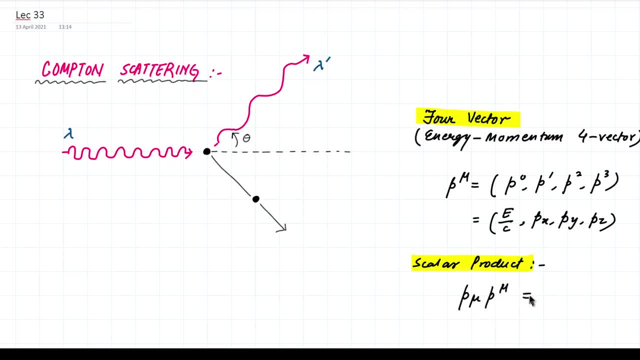 p nu is equal to how much? Do you remember Minus m naught square c square? Minus m naught square c square? Very good, Minus m naught square c square. Okay, So what will we do now? 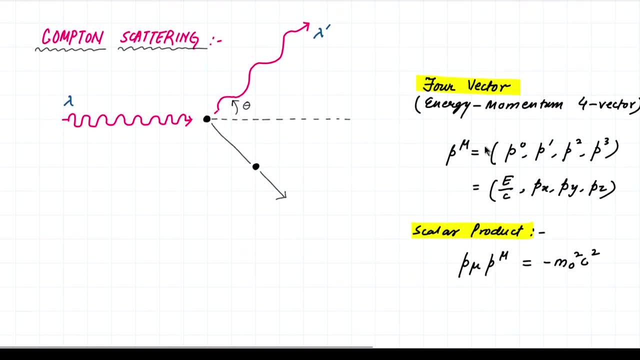 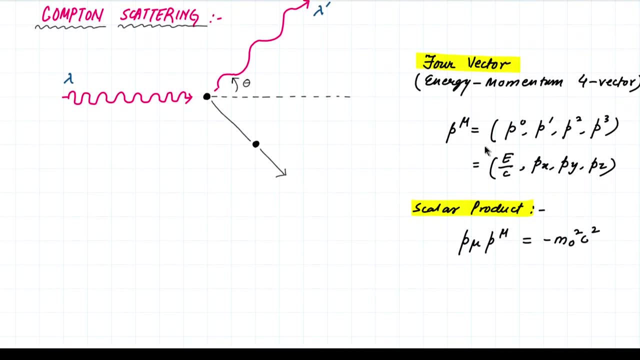 We are going to use these, This very simple concept. So, to use this very simple concept, Let's suppose that I define, before collision, both the particles. Let me define the four vectors of momentum for both the electron and the photon, before collision, Before scattering. 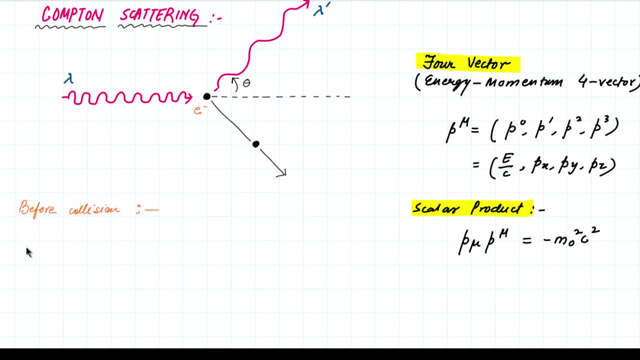 So before collision, Let's suppose Let's first talk about gamma photon. So in gamma photon I write it as p nu. Okay, Up will be mu p gamma, Okay. Okay, Let's suppose that this is the x axis. 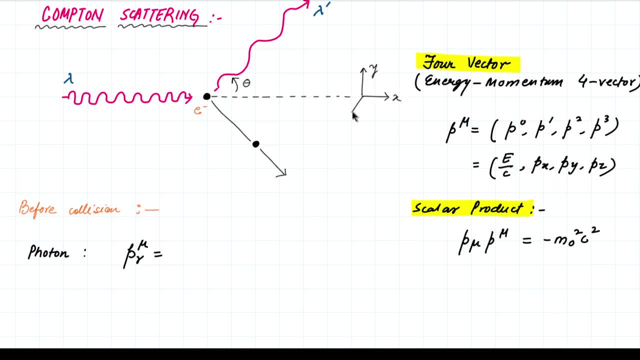 This is the y axis, Okay, And this is z axis. z axis is outside the screen, So that the scattering is more or less confirmed, More or less confined to the plane xy plane. Okay, Now can you tell me the components of the momentum for the photon? 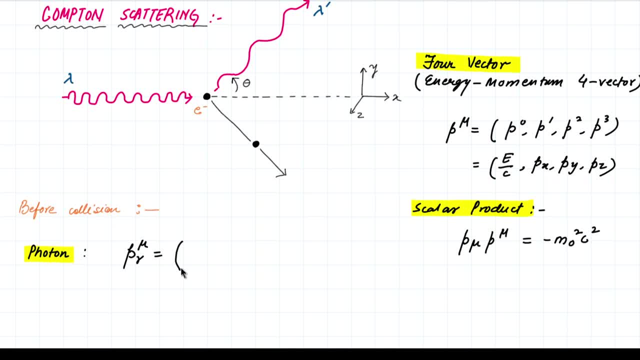 What will be the first component of the photon? What will be the first component of the photon's four vector before scattering, before collision? H by lambda, H by lambda or h nu by c. Very good, Then what will be the second component? 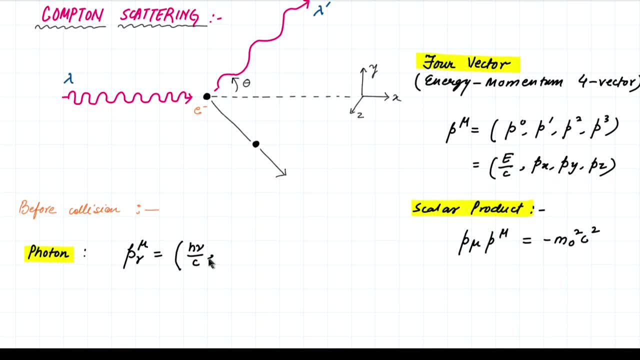 What will be the second component, ordinary momentum. what is the momentum of a photon? if your lambda is wavelength, then how much is the momentum son? how much will be p? same sir, h nu by c. i, exactly. so, that is, either we can write h upon lambda or h? nu upon c. 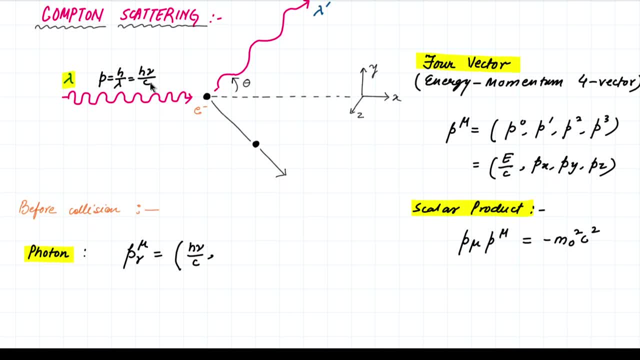 we can write the momentum of photons, is not it? what is the momentum of the photon in the x axis, h, nu upon c? third component: what would be the momentum of the photon in the y axis? zero, yeah, zero. what will be the momentum of the photon in the z axis? fourth component: 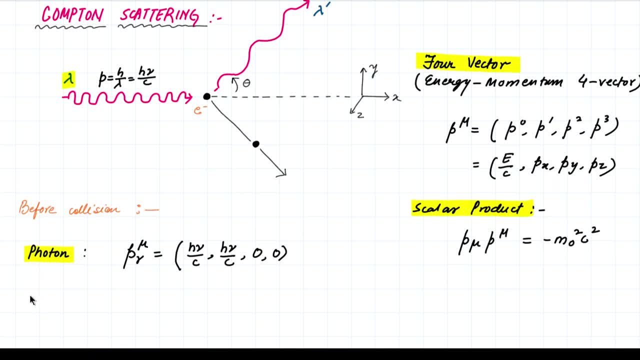 zero, zero. very good. before collision we will look at the electron p electron nu. okay, now tell me what will be the first component of electron: m0 c square by c. so the energy of rest electron is: e0 is equal to m0 c square, m0 c square upon c. 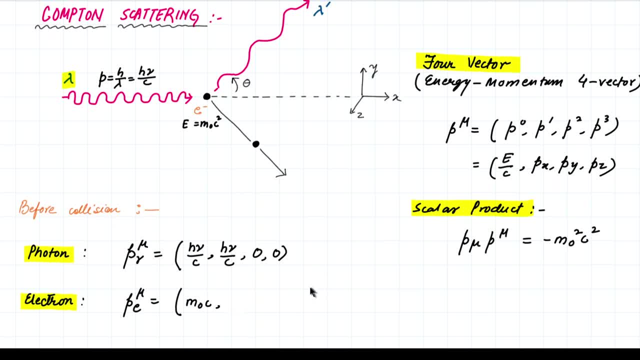 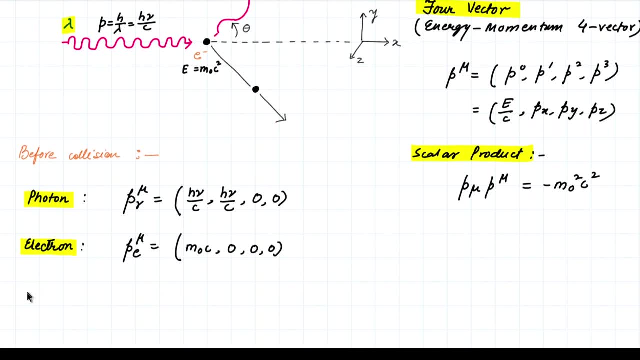 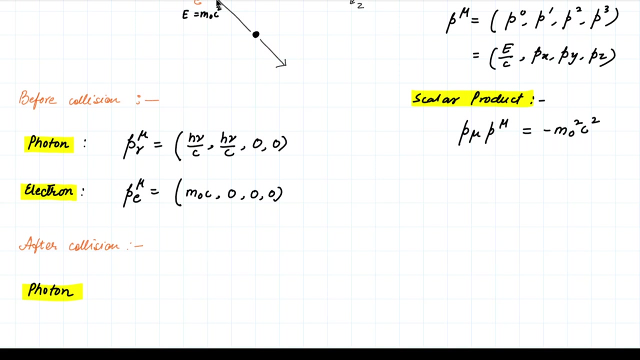 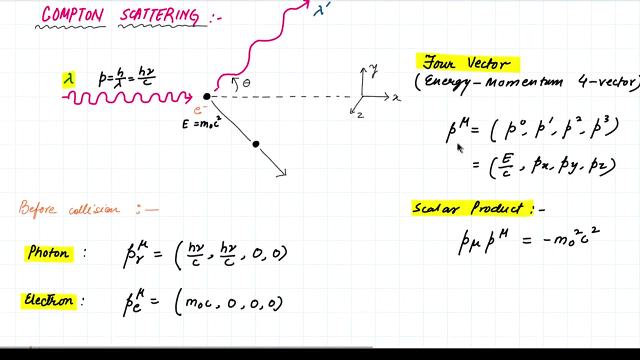 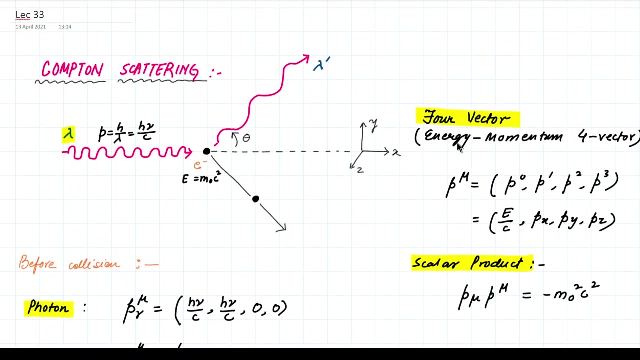 and what will be the rest of the components? all will be zero. before collision. let's look at after collision. after collision, let's look at photon. first, photon is scattered. p gamma dash nu is equal to, after scattering, what will be the first component of photon: lambda dash nu dash. 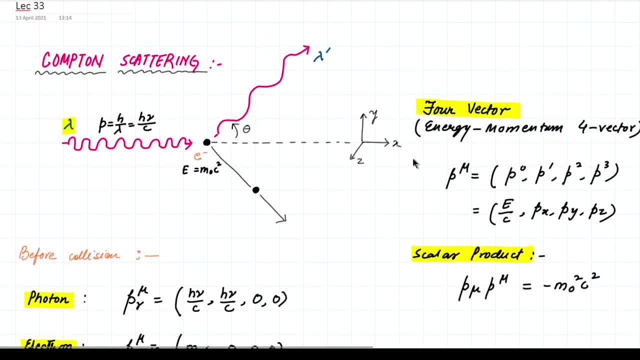 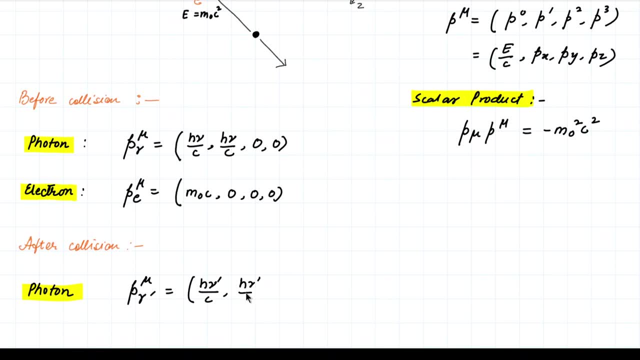 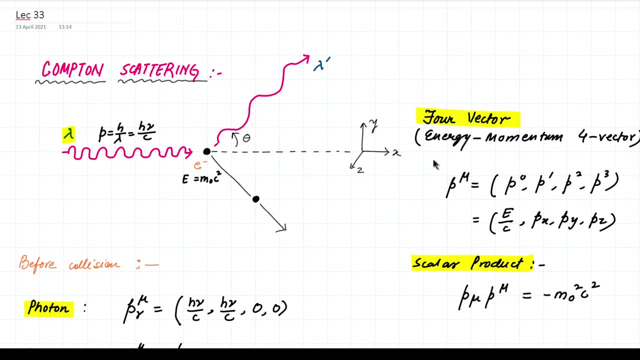 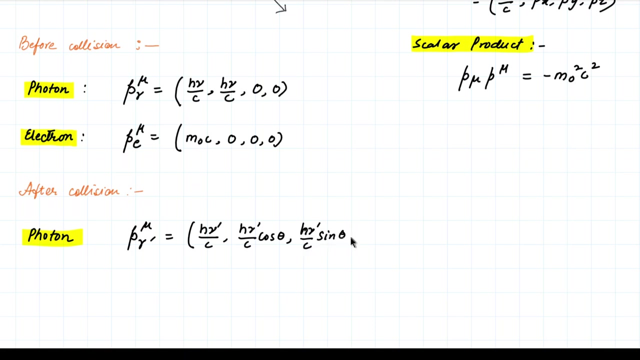 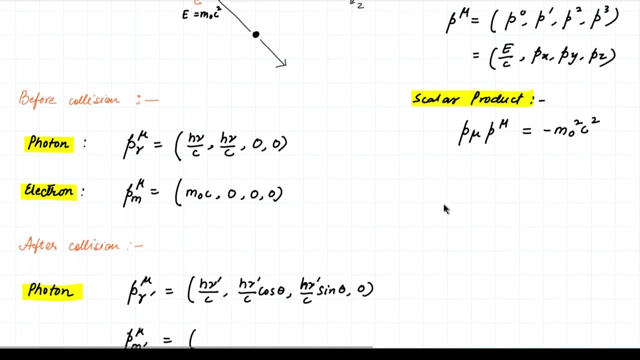 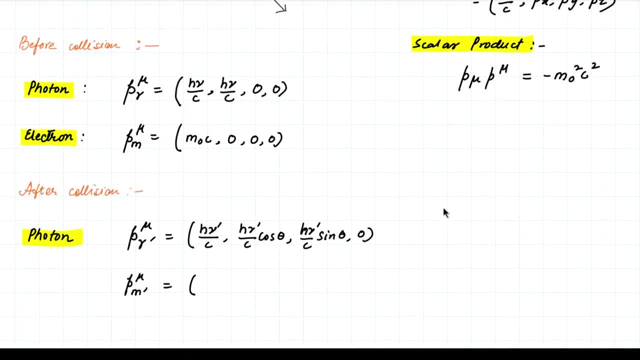 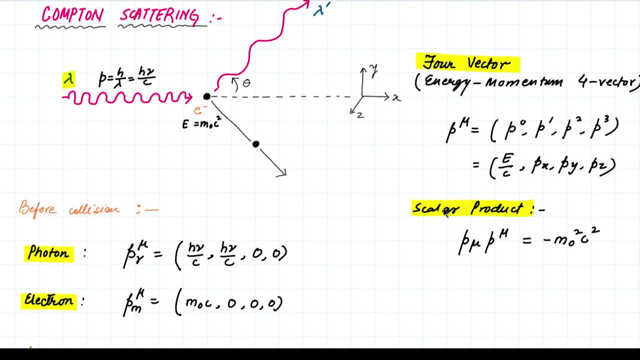 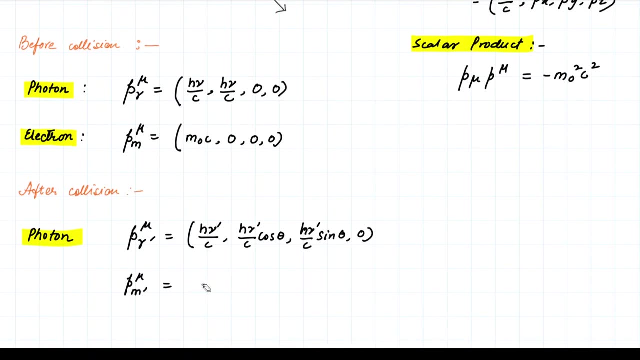 Now the thing is, if I want to write 4 vector for electron, then energy will be mc, but for momentum, then I will need this angle. let me just keep it as it is. I think I can skip this part by obtaining a relationship whatever is the momentum, because I will need phi for 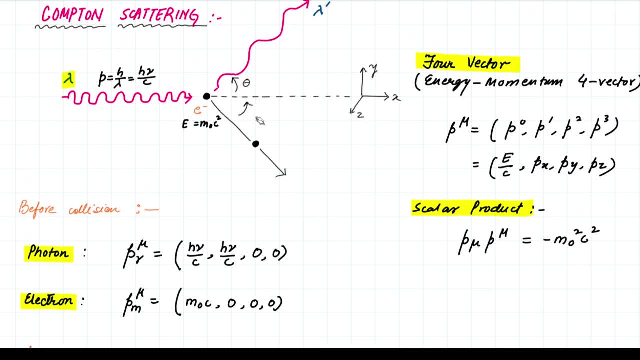 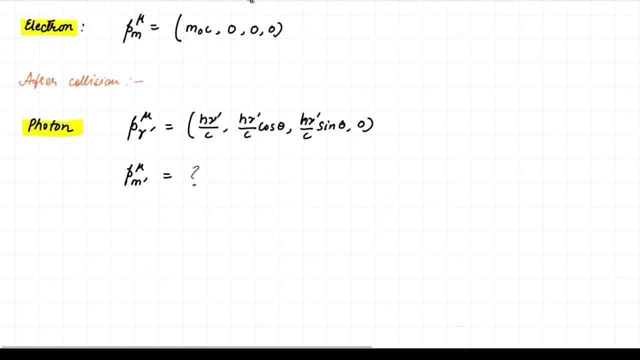 this. I don't want to figure out what phi is at the time being, so let me keep it like this. now, what did I say yesterday? that conservation of four vector momentum holds true. conservation of four vector momentum holds true. this is what I told you. so what does this mean? this? 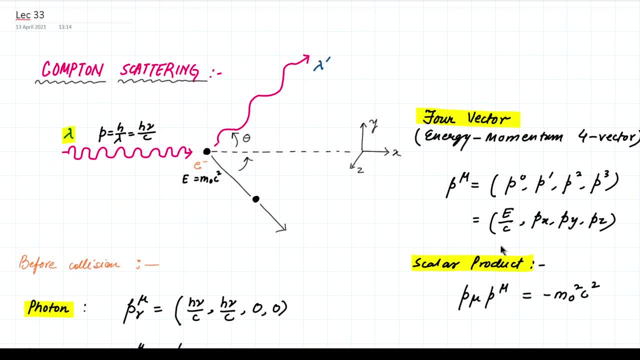 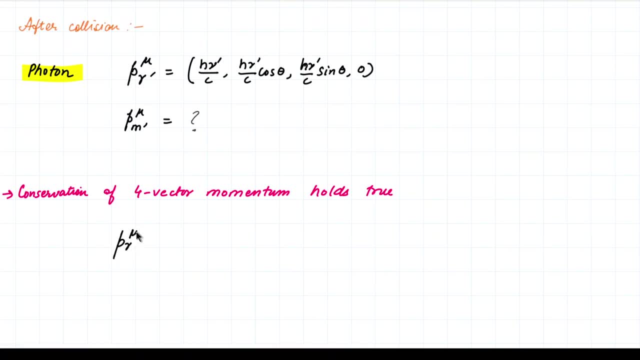 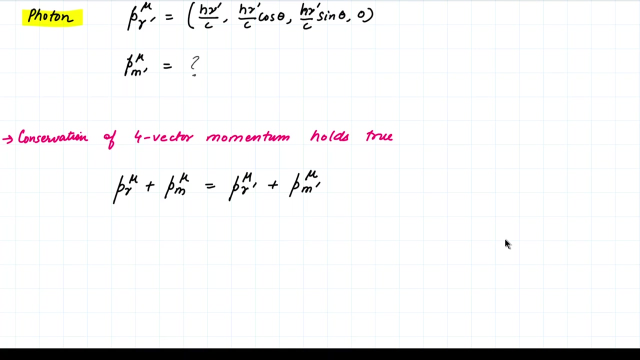 means this happened. Before collision, the total momentum is four vector momentum and after collision the four vector momentum is equal to this. this means that p gamma mu plus p m mu is equal to p gamma dash mu plus p m dash mu. this is the conservation of four vector momentum. yes, ok. 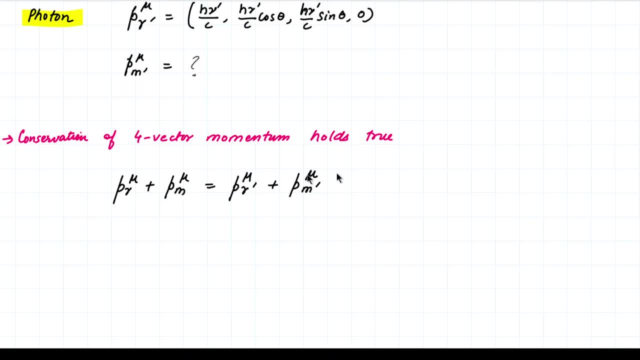 now, there are quite a lot of subscripts here, so let me just skip the mu for my calculations. The method that I will introduce to solve all the problems here is the one which is I will be using for intervention, and your Probabilist will do it. we are not going to use course. 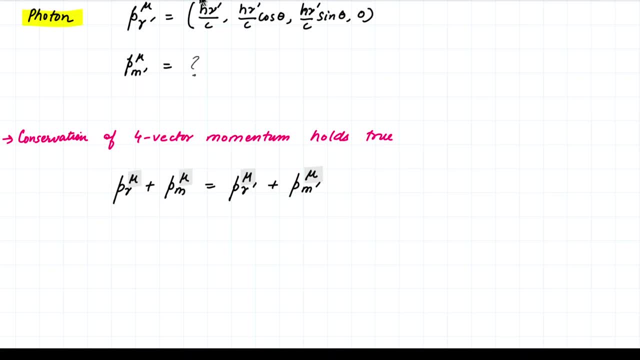 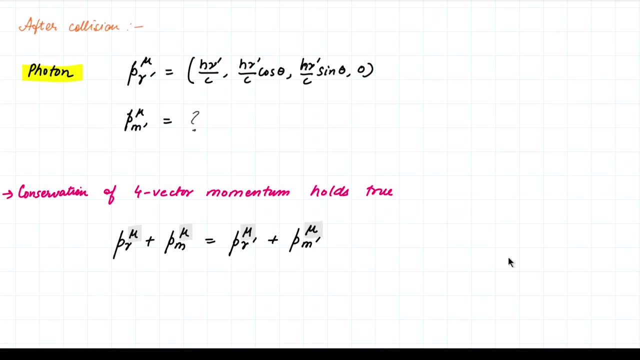 function, but it is the Maple Theory function in this which I think we got this all right. now we will go back and show you the method which is going to be used. now let me just explain to you what is this method and what is mr zebra for hunger? we are all familiar. 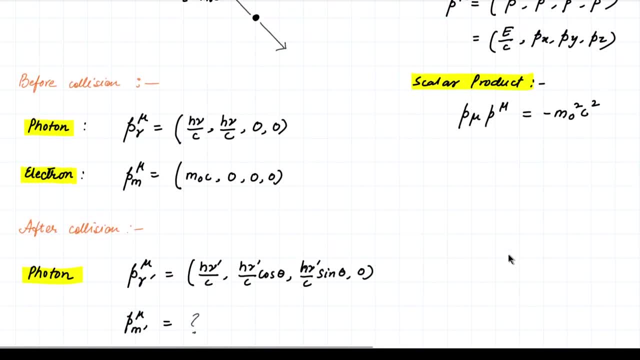 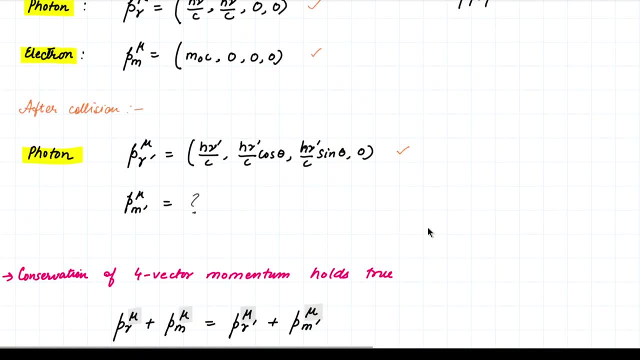 with them 70马 lake in the 4th u-25rr. we know that in protector forever as a Parkinson's, in other problems also. so what i'm going to do is here. you know this, you know this, you know this, you also know this. but let's suppose this is unknown. okay, if this is unknown, then what can? 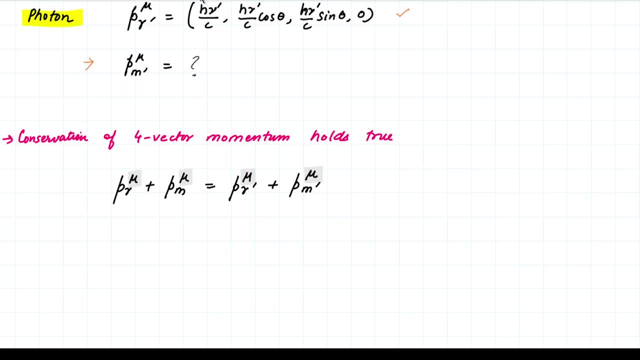 we do is we can write the unknown in terms of the known. okay, so, for example, what i can do is i can say that pm dash is equal to p gamma plus pm minus p gamma dash. you know, i have written the unknown in terms of known. now, at the time of four vector, i have written. now what i want to do is what i want to show you is that 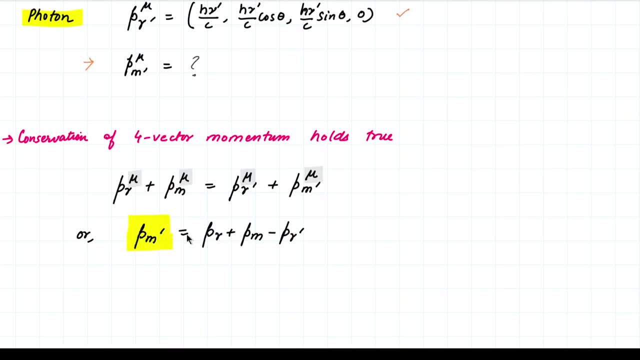 this left hand side, this is a four vector, you know, and this right hand side, this is a four vector, you know. so both are equal. the left hand side has a four vector. both of them are equal. this means that their magnitude is also equal. both of them are equal. 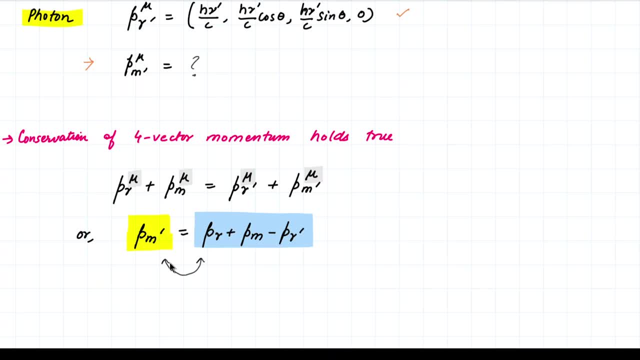 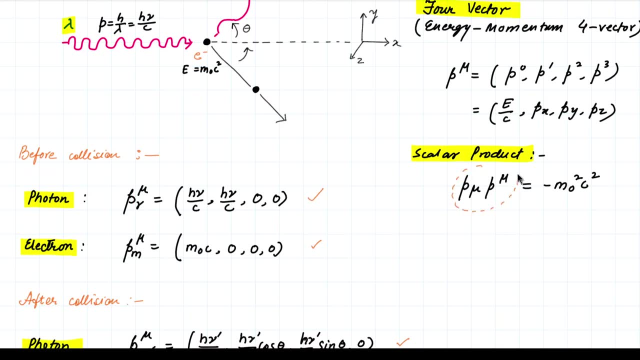 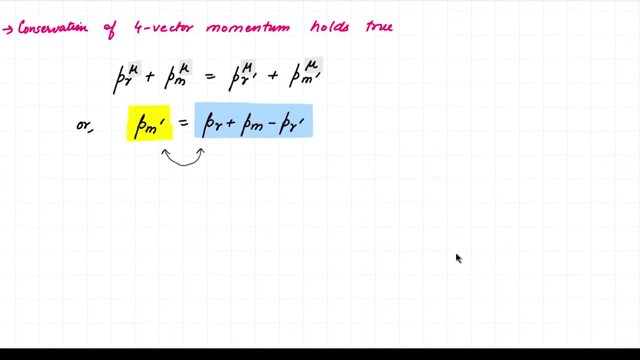 this means that their norm, their magnitude and length, is also equal. so if I take inner product of both sides, then both will be equal. are you understanding? yes, sir, if I take the inner product of this with itself, that is equal to the inner product of right hand side with itself. 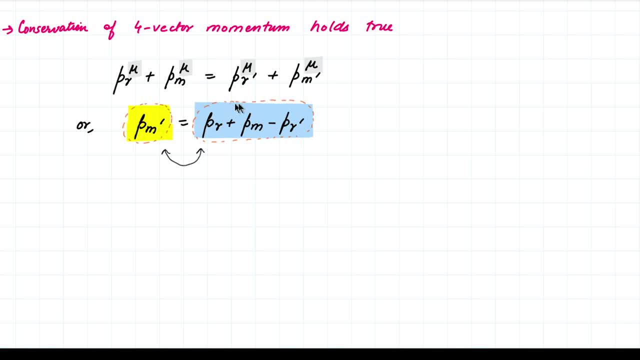 because the inner product simply signifies the square of the magnitude of the vector, the norm of the vector. so if I take inner product of both sides, then they are just nothing but equal to each other. ok, yes, sir. so what we are going to do here? what I am going to do is: 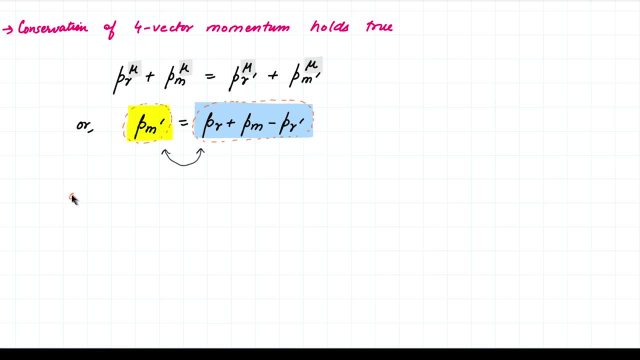 ah, ok. so what I am going to say is that let me write down p mu gamma and p mu gamma. this is done on the terms of gamma square, otherwise there will be a lot of terms. this is the inner product of this, or let's suppose p mu m. 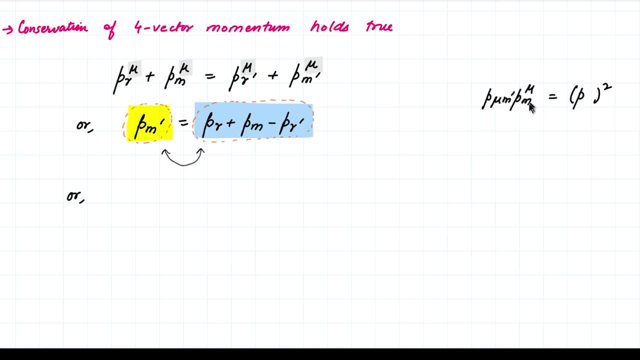 or m dash. p mu m dash is its covariant and p mu m dash is its contravariant, so p m dash square. so if I write this, then you will understand: p m dash square. this, let me say, is representing the inner product. so what I am going to do is: 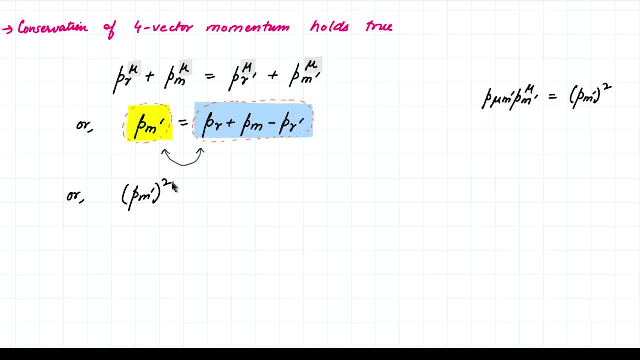 when I write this on the terms of components, then I will write a negative sign in front of the time component rest. I don't have to worry about anything else. the only thing that I need to make sure is that when I divide the components of the time component. 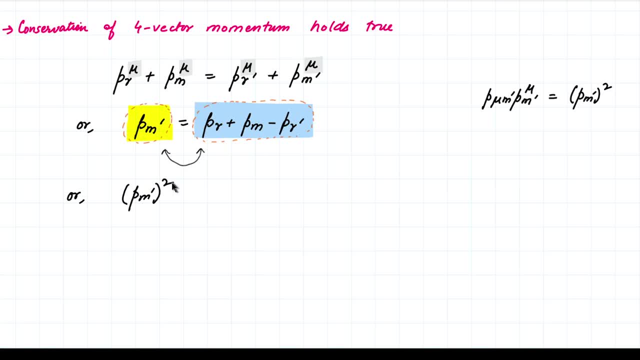 so in front of the time component I will write a negative sign. everything else is going to be the same. fine, ok, son. yes, sir. similarly, let me do this for p gamma plus p m minus p gamma dash. I will take x square. so right now I am only interested. 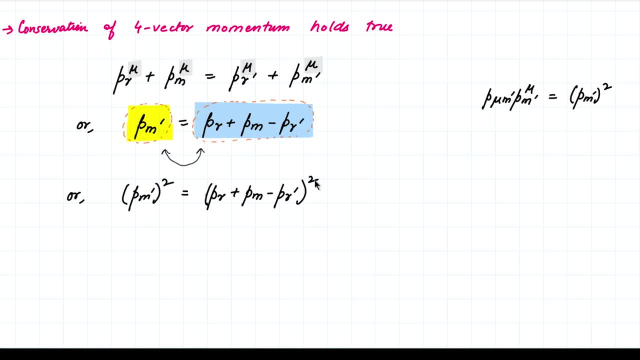 in looking at the product of the four vectors. when I separate it out, I will write a negative sign in front of the time component. so everything is going to be balanced at the very end. ok, now, what is this equal to? this is the trick. what is this equal to? 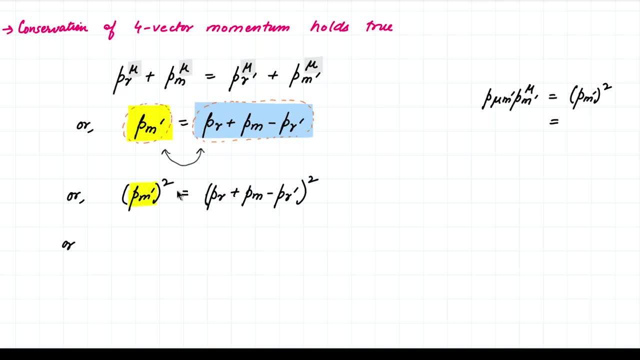 I don't know what is p m dash. it is an unknown. but I know what is the scalar product of p m dash, minus m naught, square, c square. very good, this is the trick: minus m naught, square, c square. because what I wrote here, what is this? 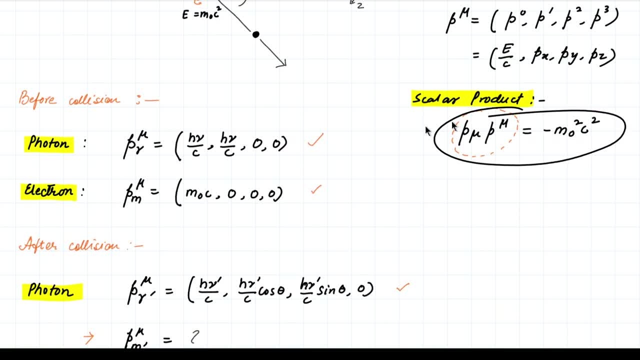 this is a any four vector. any momentum four vector is the value of any product. m naught does not depend on any particle. m naught can be different from that particle. c is the speed of light. they are constants. so any particle if the four vector of that particle is unknown. 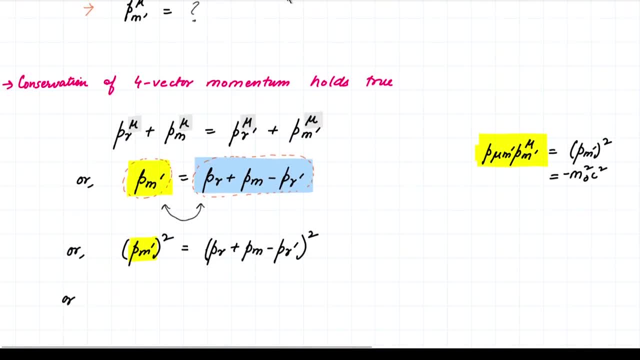 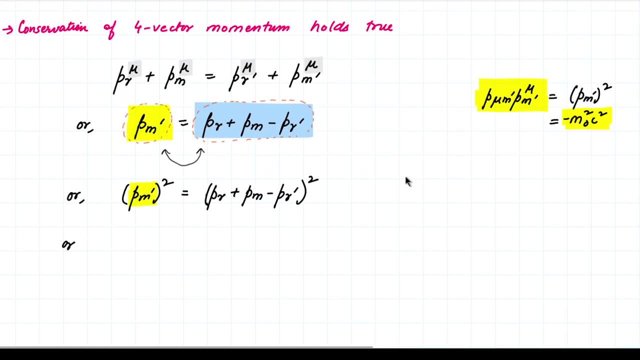 then you can take its inner product and write it in a known quantity. this is the trick. if you know this trick, now you can do everything else. what I can do is p m dash. we didn't know. p m square, c square. is this clear? this is very important. 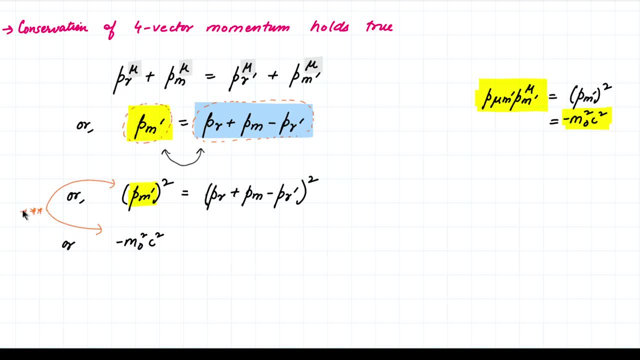 just note this. if you remember this, then all the problems will be easy. this is ok. yes, sir, rest is: let's suppose I separate it out: p gamma square, p m square. p gamma dash square plus 2 or minus 2 p m. p gamma dash square. 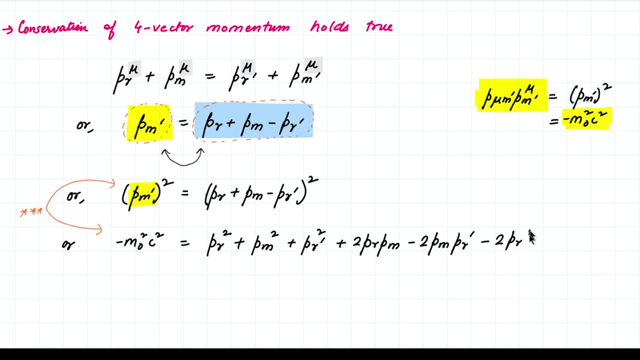 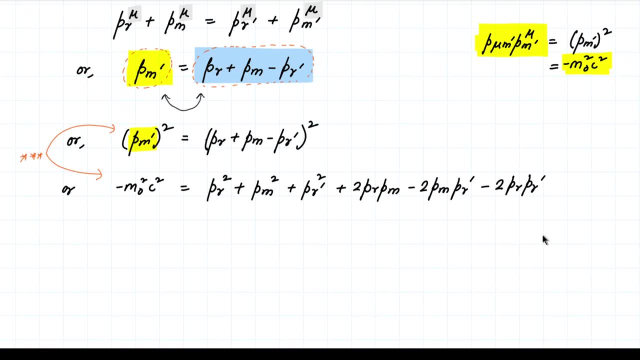 or minus 2 p, gamma, p, gamma, dash square. ok, now, now lets suppose that this is point number. point number one. now, lets suppose this is point number one. I will come back to this in a moment. What is this? What is this? What is this? Let me figure it out one by one. 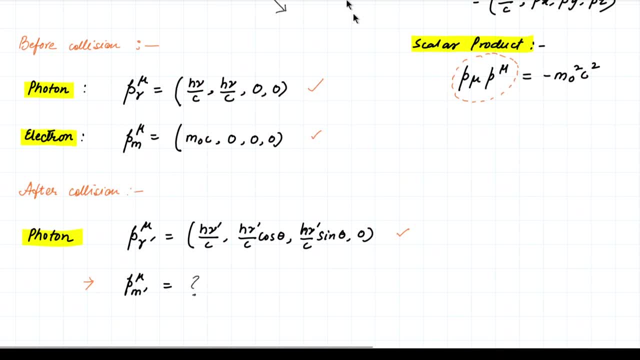 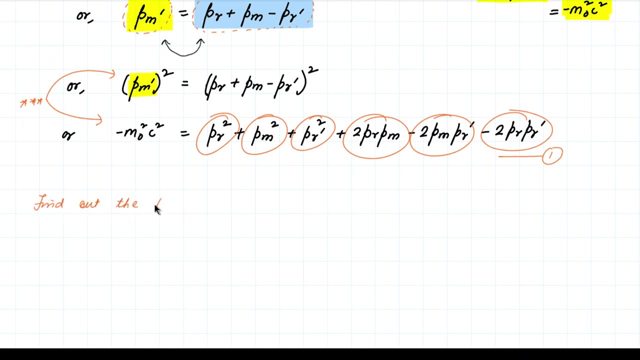 For that I already have definitions available. Let's suppose this is A, this is B and this is C. So let me figure out. find out the terms in A, find out the terms in 1 using ABC. Let's do this in detail so that you can understand what is happening. 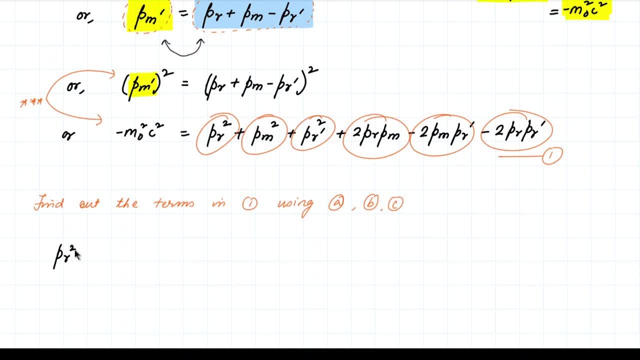 So let's take p gamma square first. So what is p gamma? p gamma is h nu by c comma, h nu by c 0, 0.. This is your h nu by c. h nu by c 0, 0.. Think of it as a dot product. 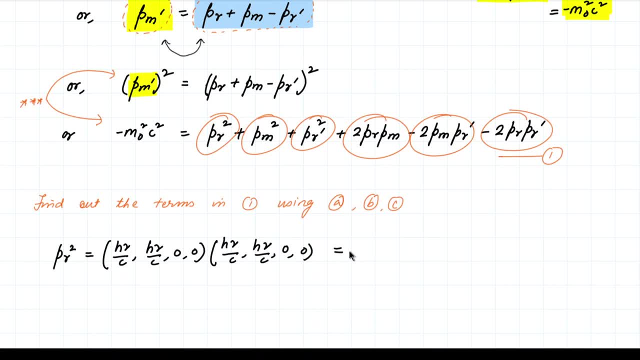 There are 4 components: dot product. What is the rule? Time component. In front of time component you have to put negative sign and nothing else. So what will happen In front of time component? h? nu by c square, I will multiply time component with time component. 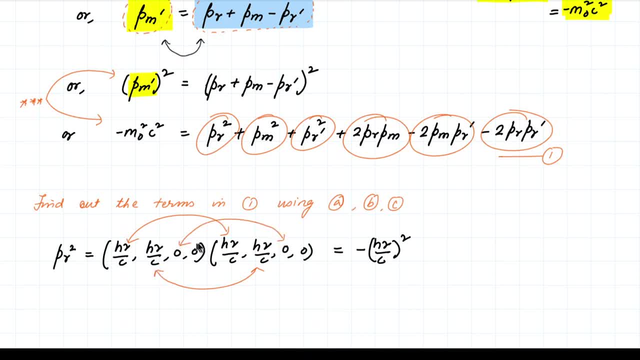 I will multiply space component with space component, Just like your dot product. What happens in dot product A, dot B is equal to AX, BX plus AY, BY, plus AZ, BZ, Right, So what is happening here? A0.. Here it is happening. 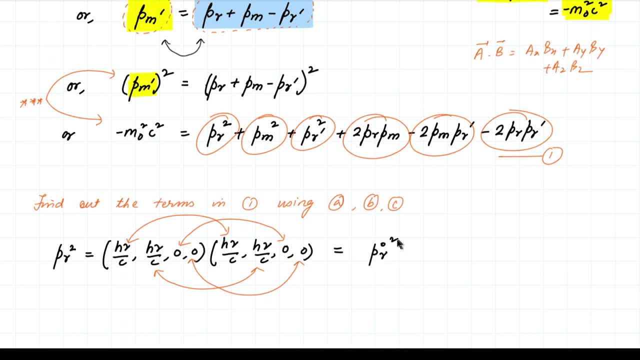 Basically p naught square minus p naught square, plus p1 square, plus p2 square plus p3 square. Are you following Yes sir, Yes sir, Ok, So first term will be done. Negative sign will be done. Keep this in mind. 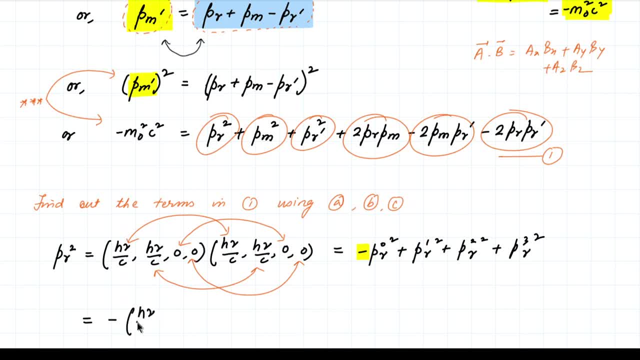 Rest is same, Minus h nu by c square. Ok, Ok, So h? nu by c square will be done. Second term will be done. h? nu by c square will be done. Plus zero square will be done. Plus zero square will be done. 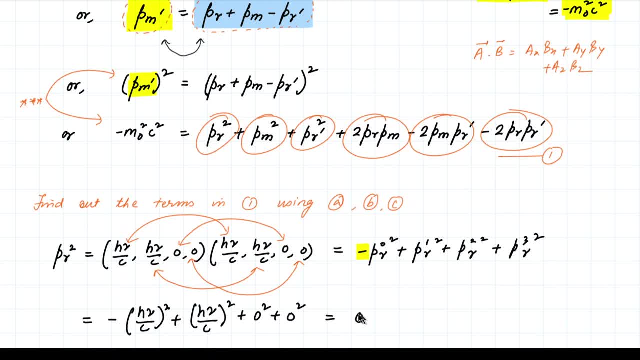 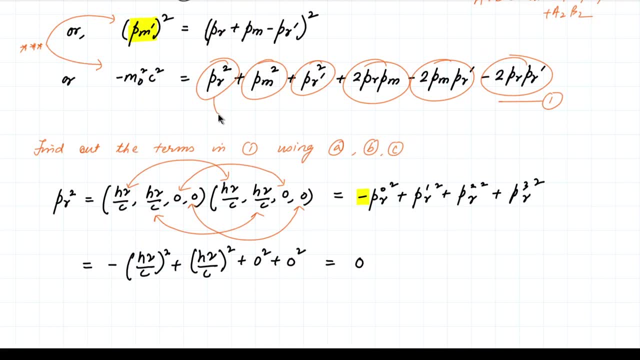 What is this? This is nothing but zero. So p gamma square will be done Your zero. First term, This will be zero. Ok, Let's look at the second term: P m square. P m square. I will simply write p m square. 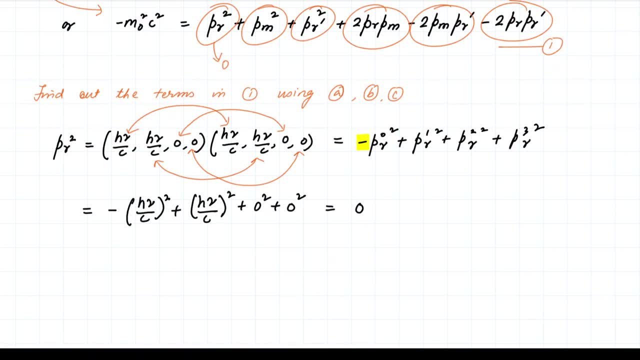 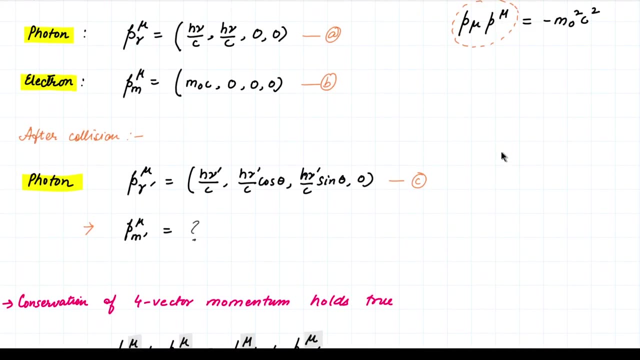 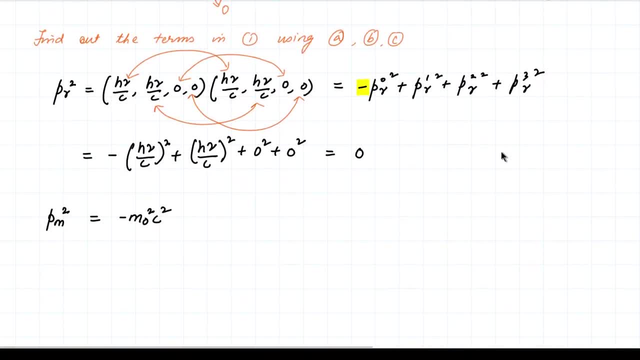 But that quantity seems aware. Minus m naught square, c square will be done. Ok, I will write the quantities too. Then it will be the same: m naught c Zero, Zero, Zero. m naught c Zero. 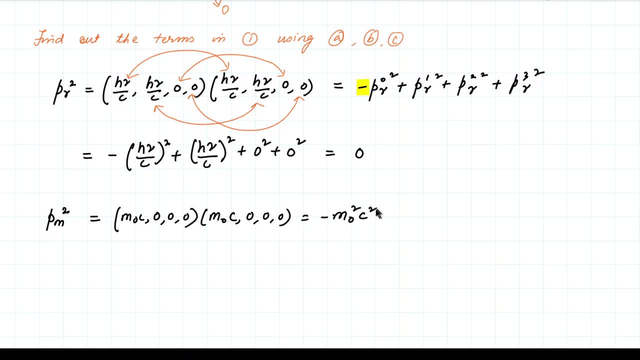 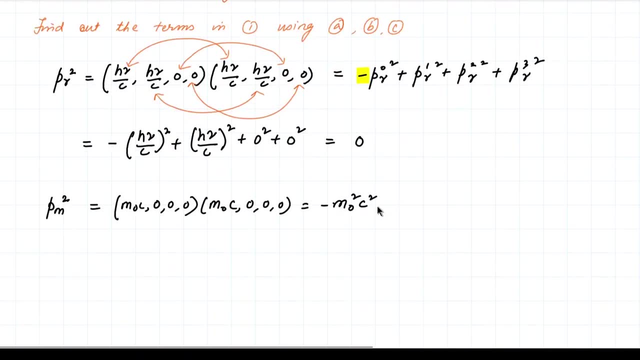 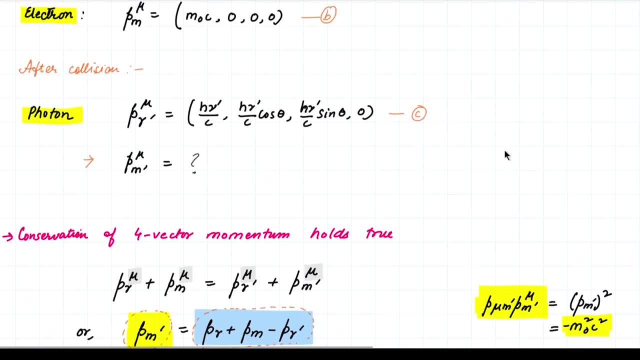 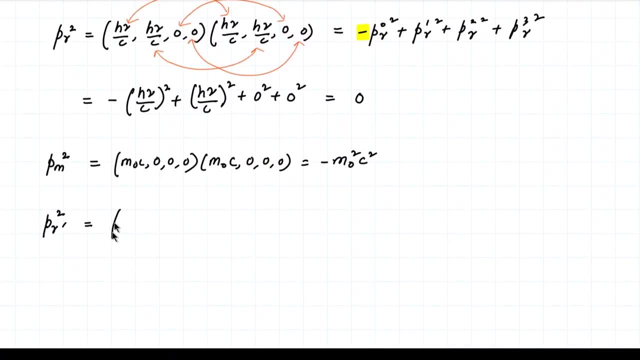 p gamma 2 dash square square. okay, so P gamma dash sky. p gamma dash a. H nu dash 1. C blue line upon Z. constant definition of upon C sine theta is 0. okay, so this is nothing but H nu dash upon C. for H nu dash upon C cos theta. for H nu dash upon C sine theta. 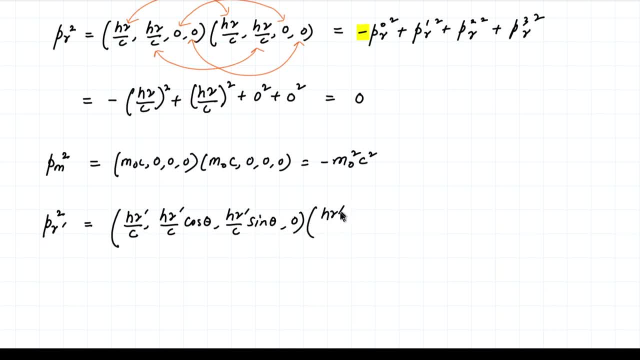 fear zero. same H nu that upon C. H nu dash upon C cos theta, for H nu dash upon C sine Theta p 0. so heeb coge mind us. H new dash upon C square plus H new dash upon C whole square, Corsica, theta plus. H new dash upon C whole square, sin square, theta plus. 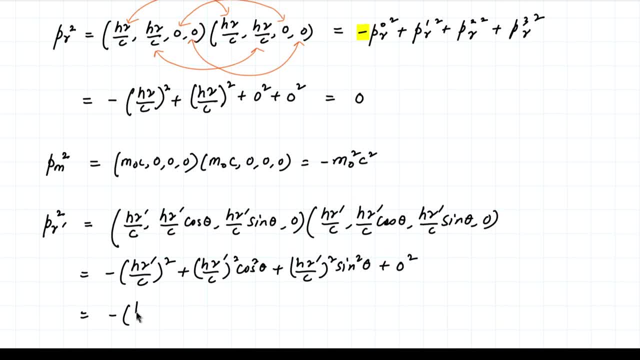 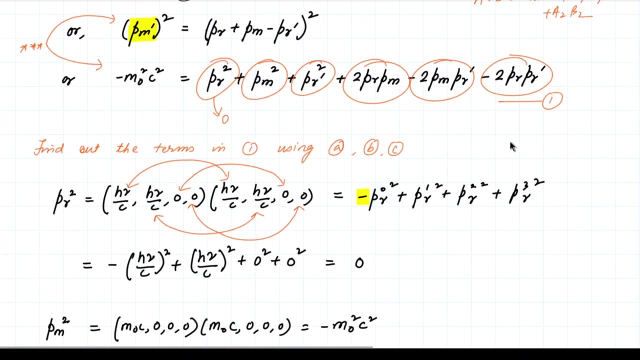 0 square. yet you have to a your mind us H- new dash upon C whole square, plus CORE square, theta, sine square, theta. here we have come on to bungalows- me it's new- dash upon C whole square. you get now we have yoga 0. so yeah, we have cup here- new dash. this is 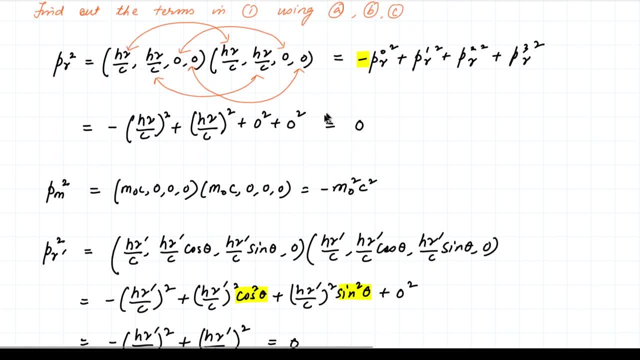 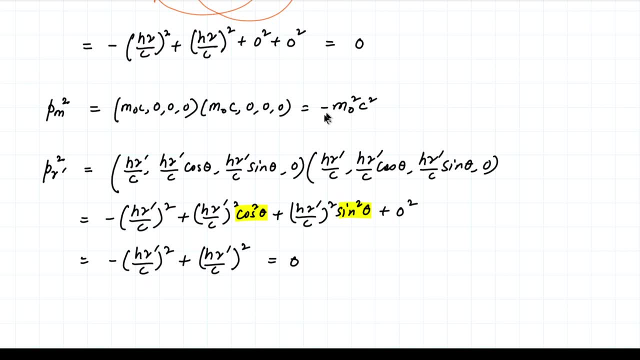 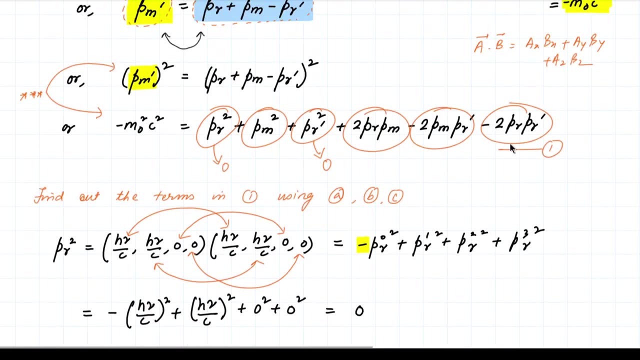 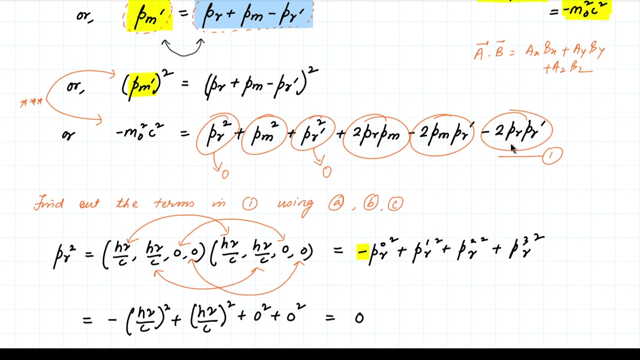 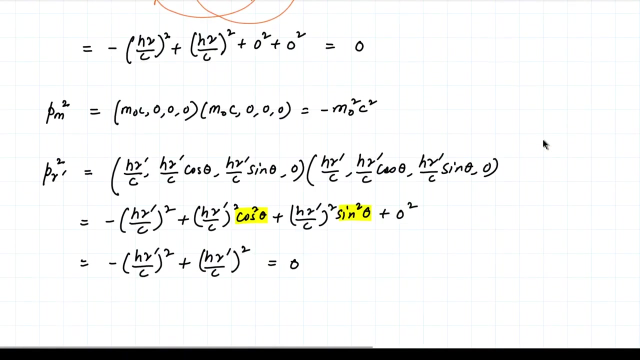 also equal to 0. fine, just as I make calculations, cut down your fear. you're following. yes, sir, okay, yes, okay. now let us look at the terms: P gamma PM. minus 2 pm p gamma dash, okay, ok. 2 p gamma 2ish minus 2pm P gamma dash, so 2. 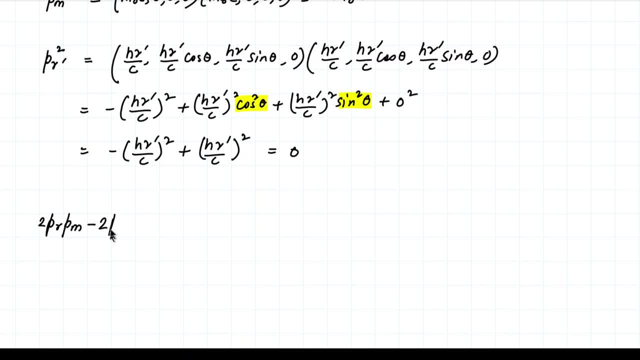 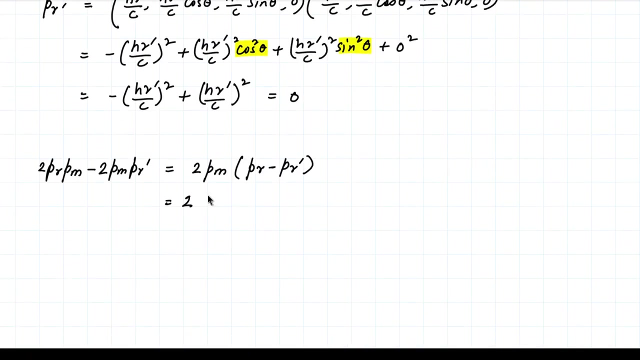 P gamma pm minus 2 pm. Flor Madel's huh to be gamma pm master, pmp gamma dash. okay, so what is this? this is equal to 2 pm. come bar Nicola thing. but yeah, P gamma minus P gamma dash, TK 2 pm pm. k, happy m is just, I'm not C. 0 0, 0 yeah. 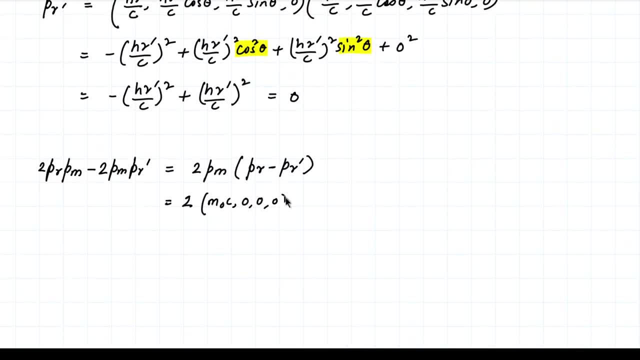 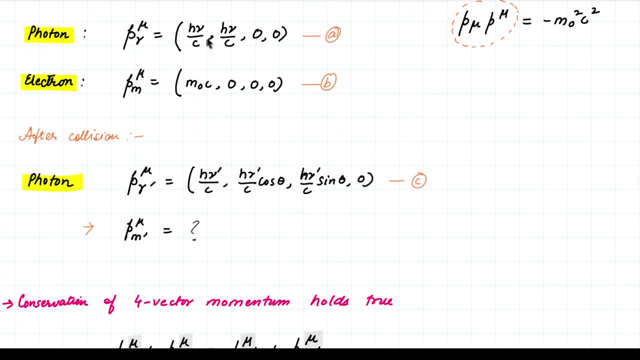 APCA and not C 0, 0, 0 p gamma minus P gamma dash. kiya hai p gamma minus P gamma dash gamma. may it's new by C term a happy h new dash by C cos theta or h new dash by C sine theta. a sub terms: a dollar minus karunga to minus karunga to. 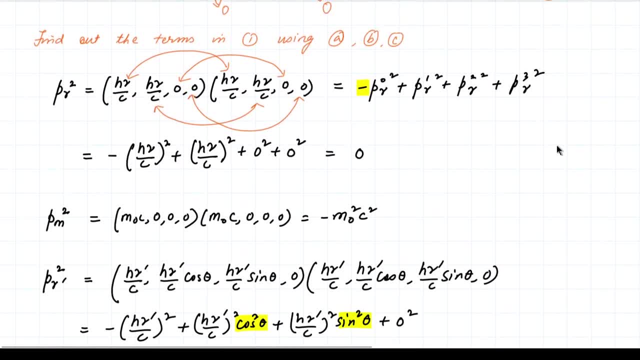 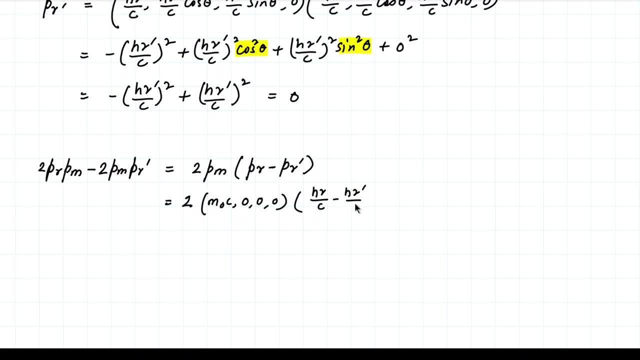 a jaga it's new by C minus h. new dash by C Palo Tomo a happy h new upon C minus h. new dash upon C first term. do certain over h new upon C minus h new dash upon C cos theta second term over h new upon C, make second of the zero sorry third. 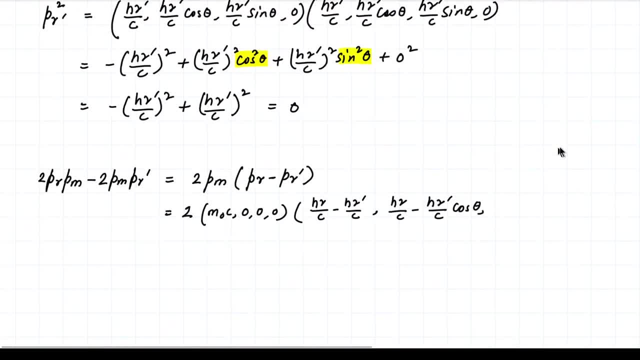 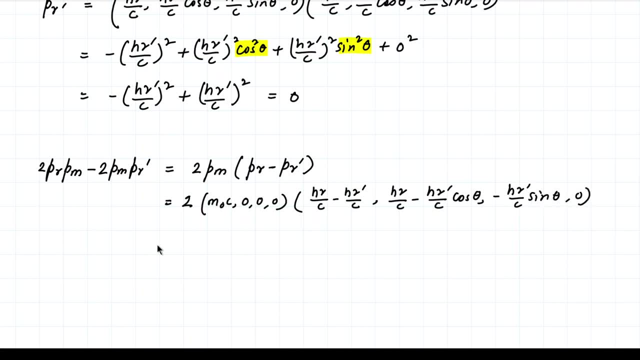 term kit naab is 0 and 0 minus h new dash by C sine theta. so 0 minus h new dash upon C sine theta. last term is 0. okay, so this is equal to you have a top cause. how much may I go yet? second, third, fourth term: zero. over here. so this is equal to here. you will understand that the second, third, fourth term will be zero. so this is equal to here. you will understand that the second, third term will be zero. so this is equal to which will go ever cause, which is fall our top growing, which is not going to happen. 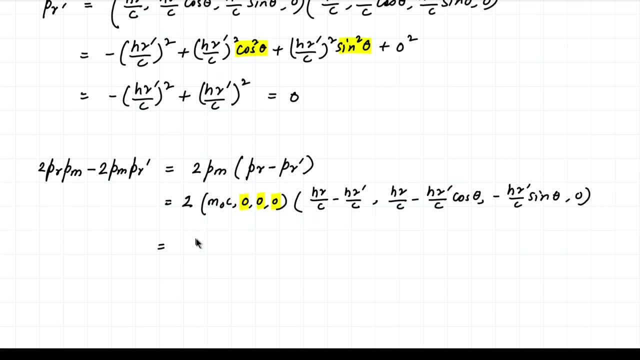 which is also not going take very many more times, whereas first term control, which is also ava real thing, does in the case of this one. in this case, but the first term control, j is equal to the other way, how to do is to bring over to starting E, to the order capital over J, since we know the하on també a. 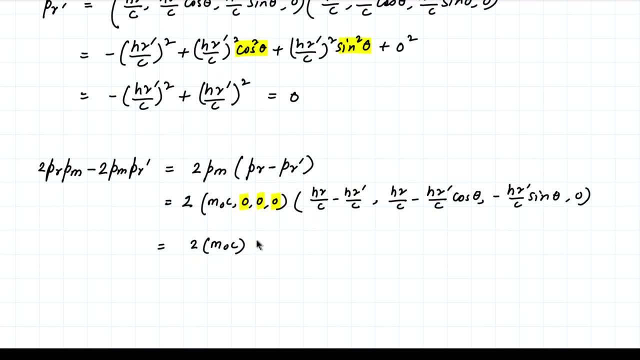 bazaar. just try to solve if I were to combine it with k? u now n ca 1c, non c. mu minus mu dash. minus 2 H M naught, mu minus mu dash. okay, yeah, yeah, last term, let's find out the last term. minus 2 gamma, 2, gamma dash. let's find out the. 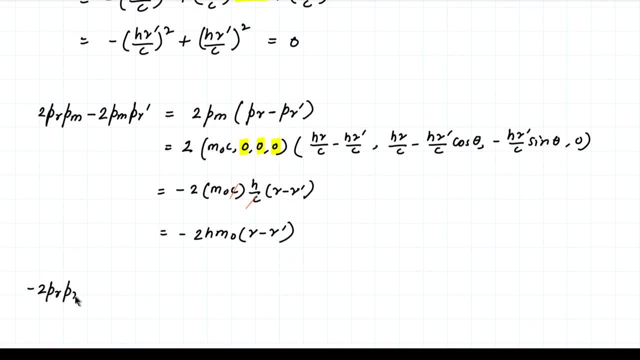 last term, minus 2 P gamma. P gamma dash. P gamma, 2 gamma dash. minus 2 P gamma. what is gamma? is H mu upon C? H mu upon C, 0, 0 gamma dash? what is H mu dash upon C? H mu dash upon C? cos theta. H mu dash upon C? sine theta and 0. 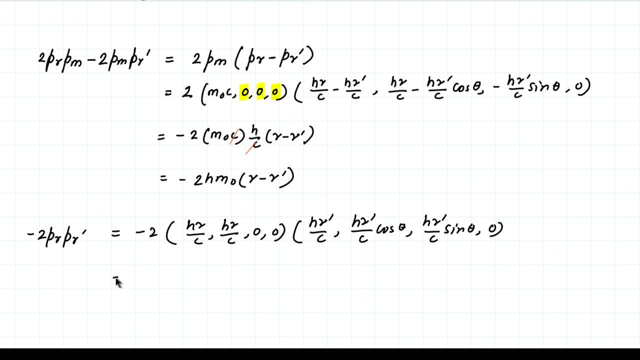 so if we sort out this, then what will come? if we sort out this, then it will come. let's keep minus 2 out. the first term is minus H mu by C. H mu dash by C right. the second term is H mu by C and H mu dash by C cos theta. then the third and 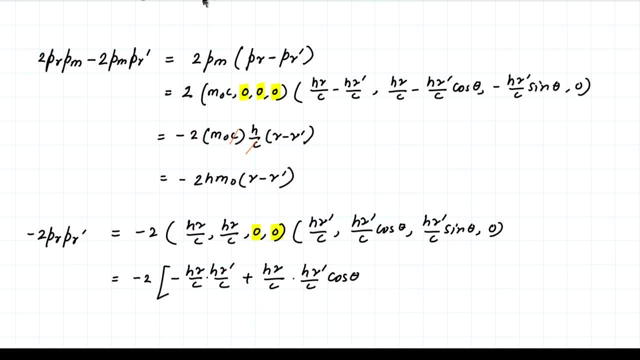 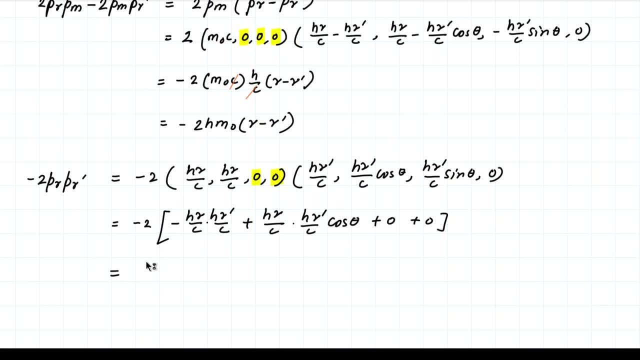 fourth will be 0 plus 0 plus 0. so this is your 2 H by. let's take out H mu by C, H mu dash upon C. also, let's take out what is left. this will be minus minus plus and this will be minus. then 1 minus cos theta. 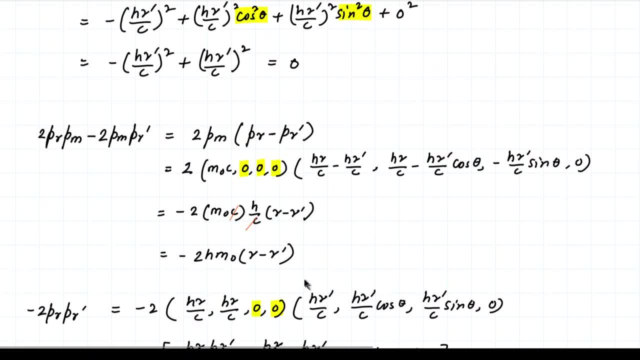 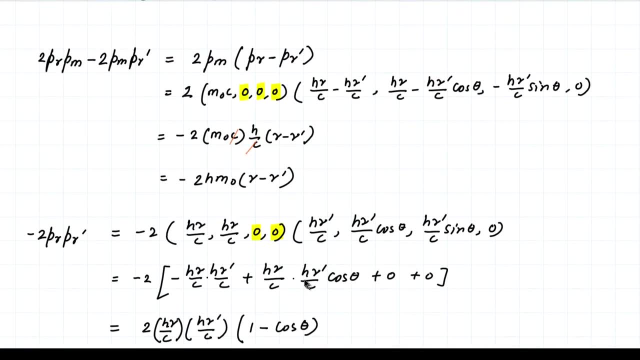 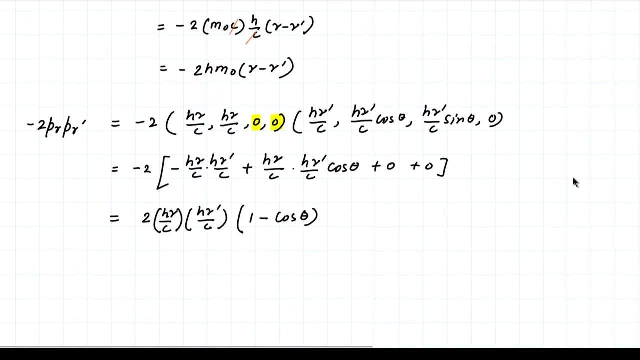 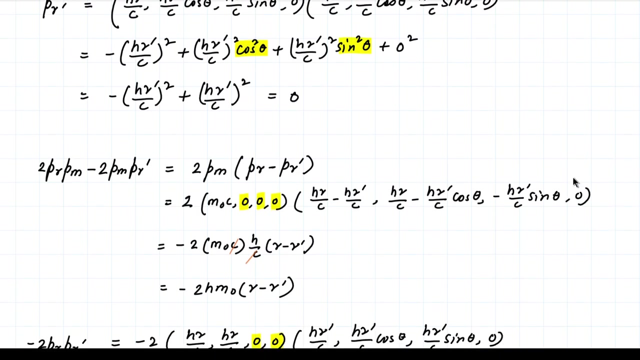 this is 1 minus cos theta. okay. okay, let us plug these values here. till here you have been able to follow the calculations. yes, sir, only component wise multiplications are happening here, so let us plug these values. yes, tell me, sir, here we have put vector for product which is M minus M, naught C square in the momentum. 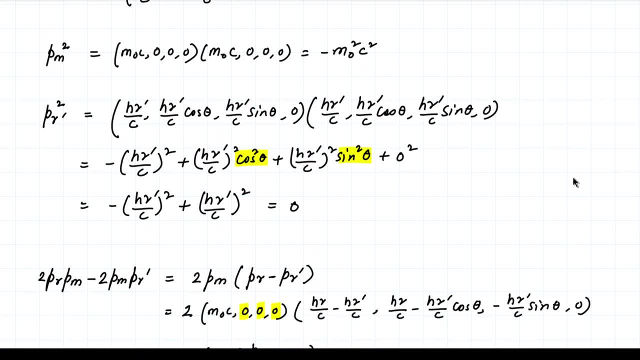 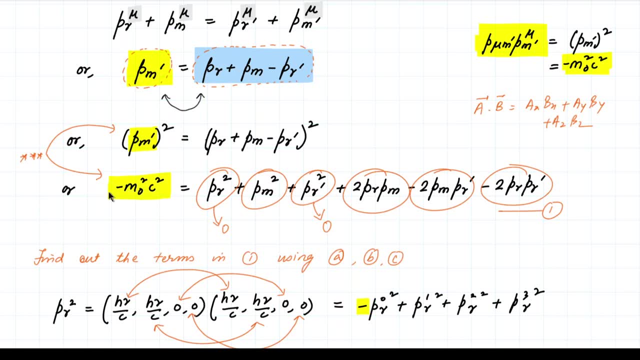 where we have put it for PM: dash square. yes, this minus M, naught C square. yes, sir, yes, sir. now, sir, when we are doing this for Gamma also, this is coming 0 and this is coming back for M. so why is it happening like this? 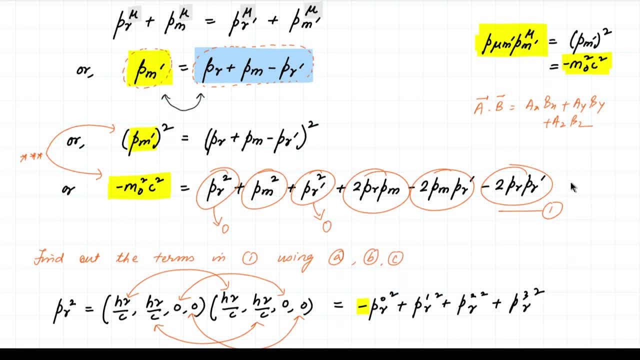 because of photon's res mass is 0. so this is valid for the particles? no, no, this is also valid for photon, but for photon M naught is 0. ok, Gamma means photon, right. for photon also, it is minus M naught square, C square, but M naught is 0 for a photon. 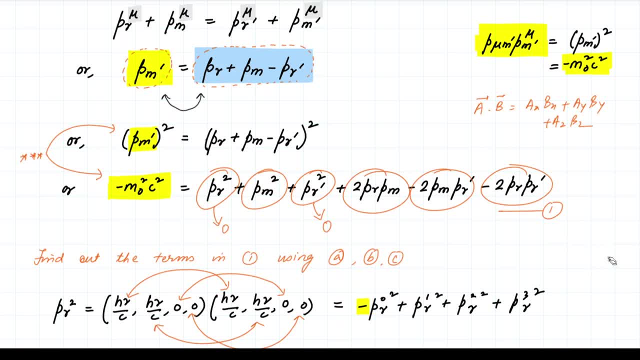 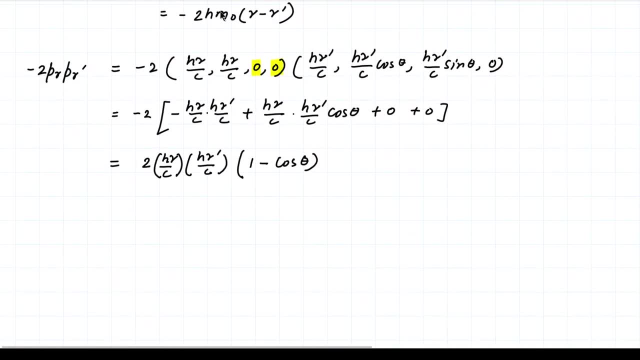 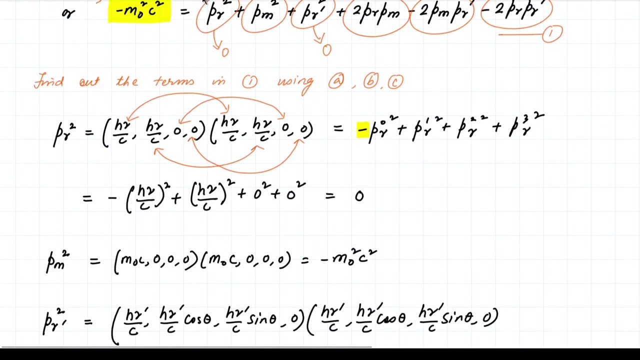 because this is res mass. res mass is 0 for a photon. so let us plug these values in equation number one. okay, let's plug the above values. okay, the equation one you will get up a little minus M naught. square C square minus M naught. 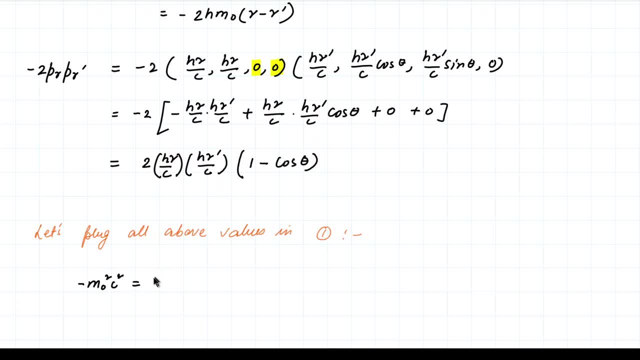 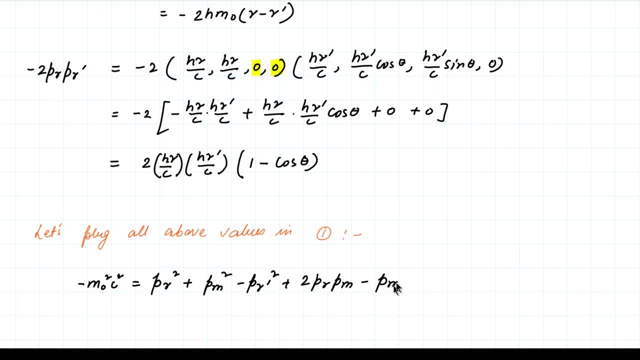 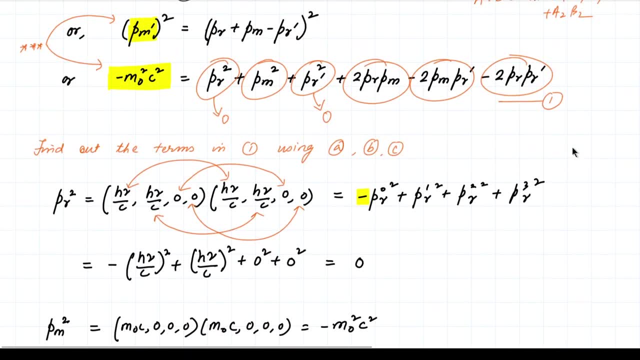 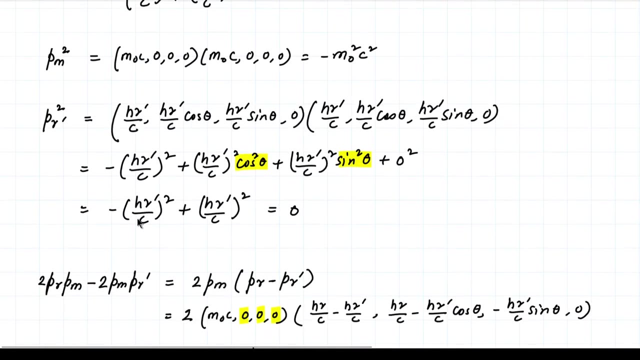 minus 2 P gamma P M. minus 2 P M P gamma dash. minus 2 P gamma P gamma dash. put a equation male idea now. so the first term P gamma square is equal to 0 and the third term is also equal to 0 and second term is minus M naught square C square. first term is 0, second. 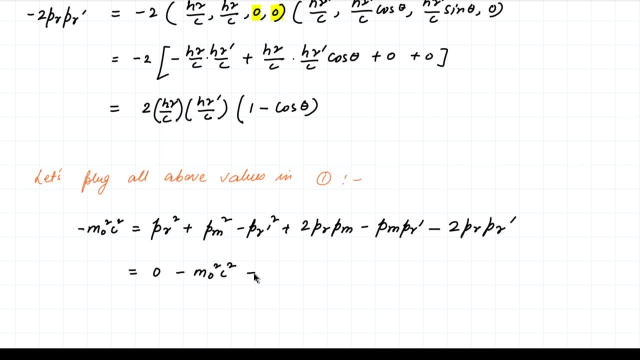 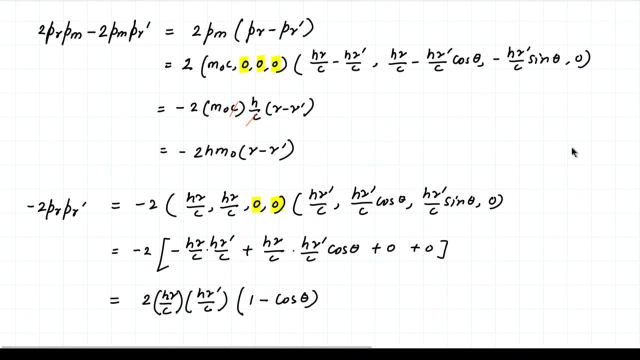 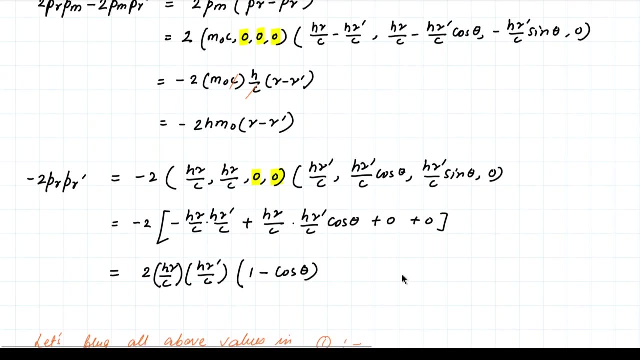 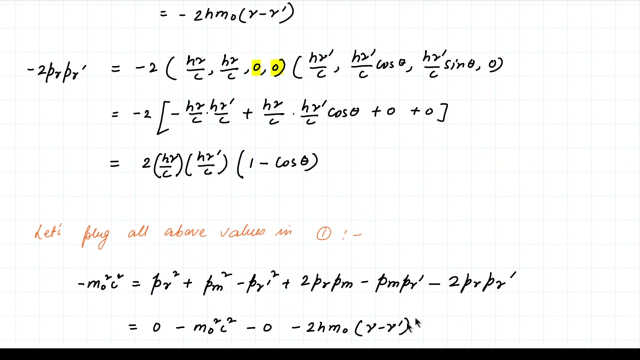 term is minus M naught square C square, and third term is also equal to 0. fourth term is coming from here: minus 2 H M naught gamma. minus gamma dash, plus plus, which I have, the minus 2 H M naught gamma. sorry, nu minus nu dash, nu minus nu dash. nu minus nu dash, or the last term. 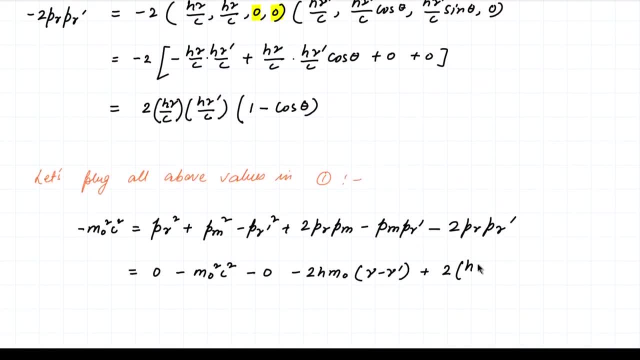 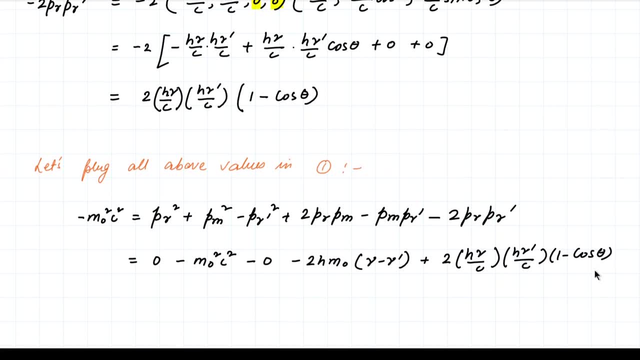 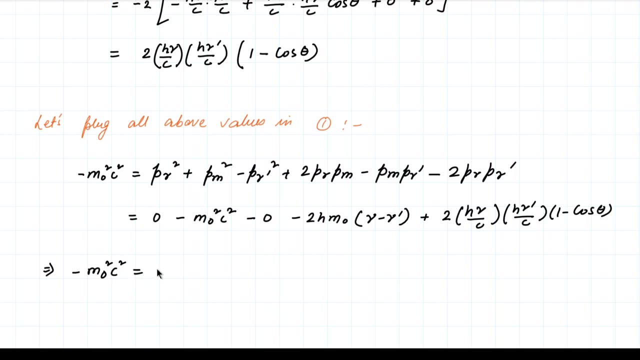 oh yeah, happy plus 2. H nu upon C, H nu dash upon C. 1 minus cos Theta. so finally this becomes minus M naught square. C square is. so finally this becomes minus M naught square. C square is solid minus. cancel out, yes, then finally. 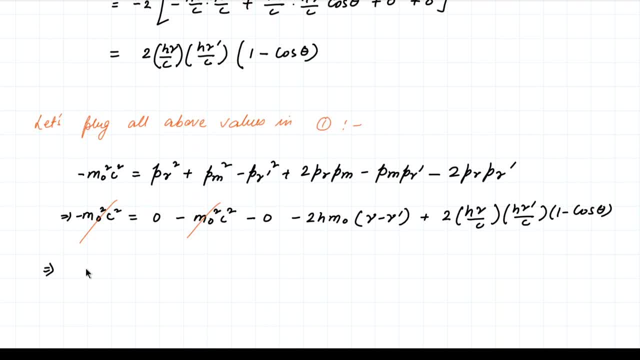 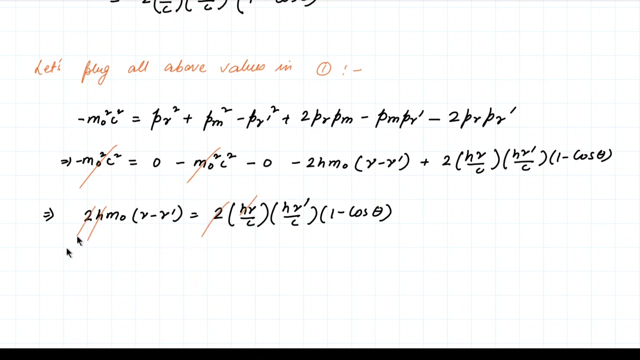 ah, HM, not new minus new. dash is equal to 2h. new by C H. new dash upon C: 1 minus cos theta. here your HH cancel to to cancel and new. can we write C is equal to new lambda. we can write C is equal to C upon lambda. 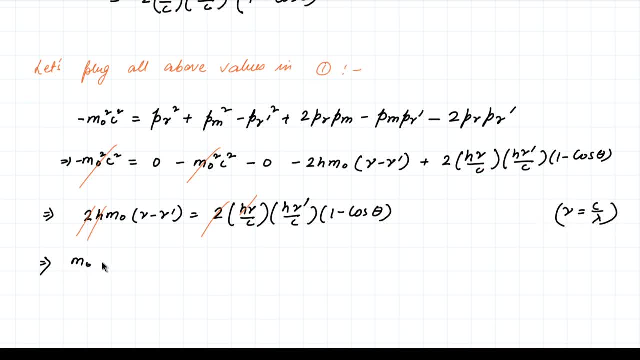 so M not C upon 1 by lambda minus 1 by lambda dash is equal to new upon C will be 1 by lambda and 1 by H- sorry H. 1 by lambda lambda dash and 1 minus cos theta. so even Java lambda lambda dash. 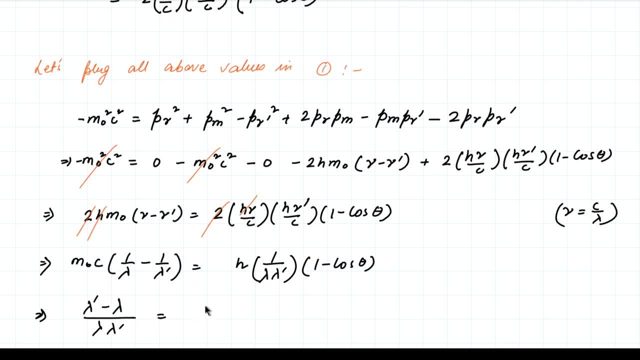 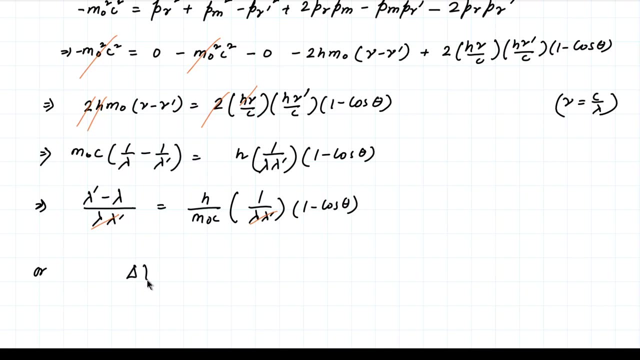 lambda dash minus lambda is equal to H upon M, not C 1 by lambda lambda dash 1 minus cos theta, the yo gap could cancel. finally you end up getting or delta lambda, which is the shift in the wavelength of the scattered radiation from the incident radiation, is equal to the in scattered radiation wavelength. 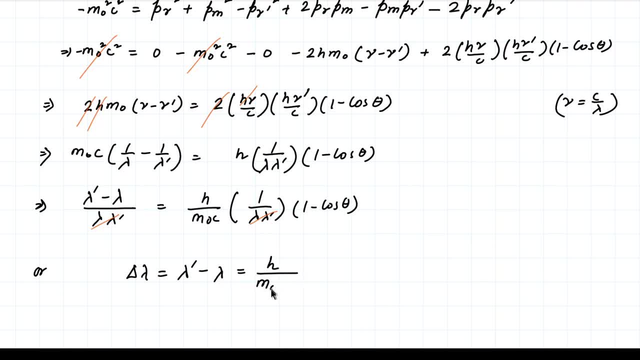 minus the incident radiation wavelength is equal to H upon M, not C. 1 minus cos theta, where H is the Planck's constant, M not is the rest mass of the electron theta is a scattering angle and C is the speed of light. this is the Compton form. 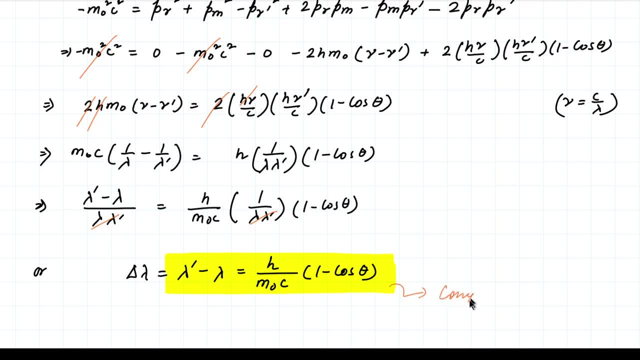 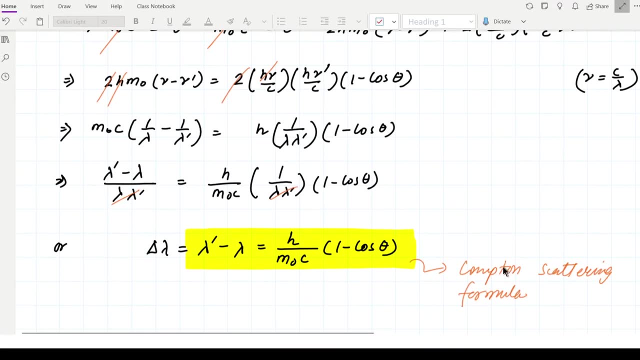 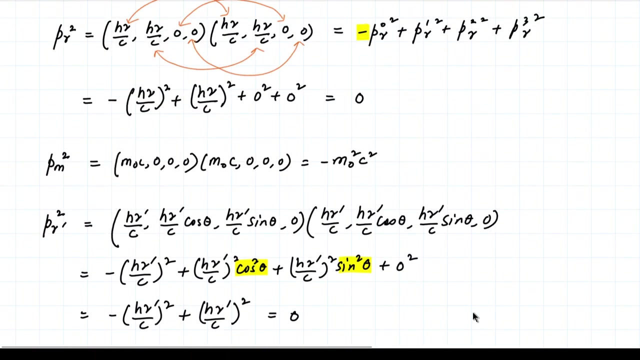 Compton formula. Compton scattering formula. now I know that you know how to solve the problem of Compton effect, but the main purpose of the lecture was to show you how to do it using four vectors, because once you understand the idea of how to do it using four vectors, you can. 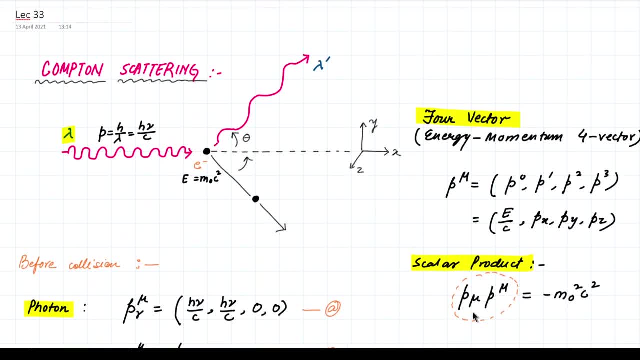 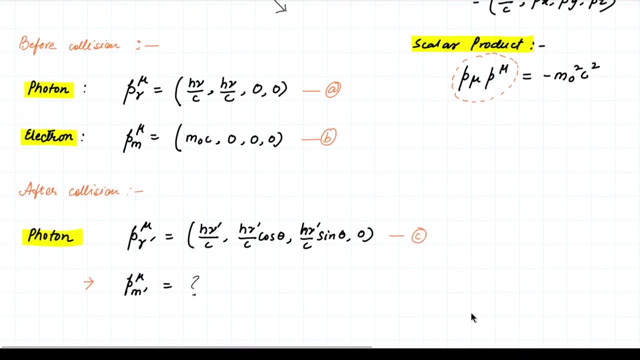 also borrow this idea with two other problems. so we have family, can't care. salt the number before scattering or before after scattering. Haman a dono. but because what on electron dono ki four vector momentum, lit the a few who сказал conservation of four men or vector momentum come in equation, lit the. 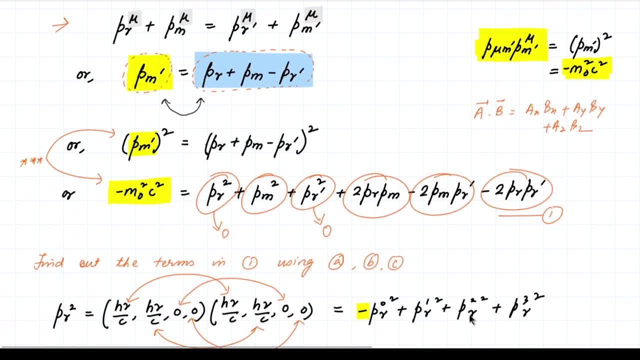 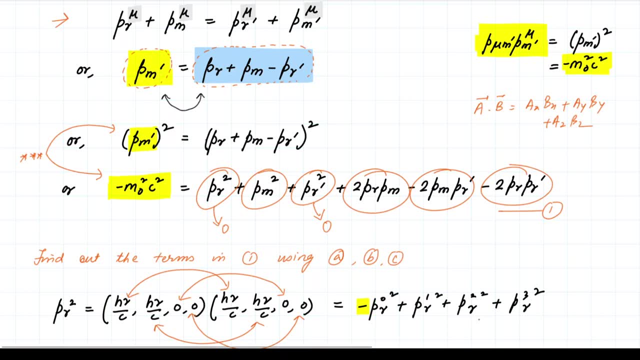 eye Joe. yet huh feel lick or key firm in a Dono side car normal area. Dono side kind of a taejo unknown thought whose Kajal norm heavy known, oh yeah. or Bucky casual Tom say, oh many known of you say, find out earlier. 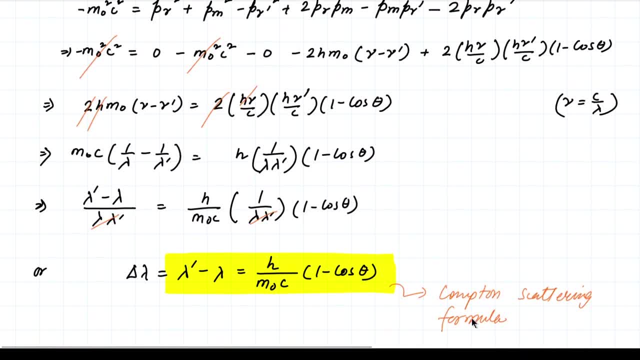 substitute, cut the occurred to he. I end up getting this equation mathematically. solve karte, and I'm getting this particular result. that's it. it's a good out, a tissue, quick question, any doubt? you have any question? you haven't some questions, I guess? yes, no doubt, yes, okay. 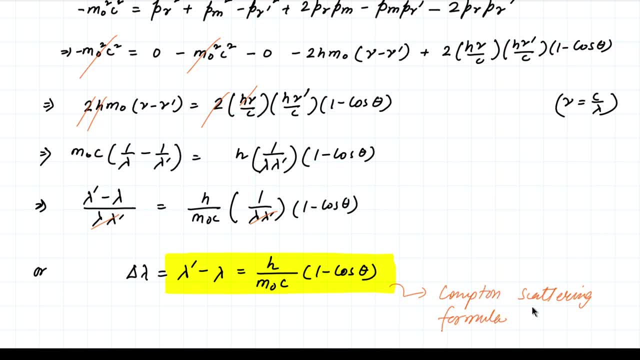 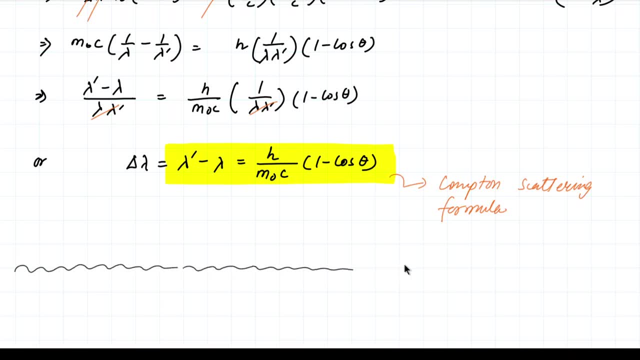 okay, I have 15 minutes. I want to do another problem, but okay, in the next class I'll be doing how to figure out the problem of how unstable decay particles decay. mostly what happens is four vectors are used in particle physics, high energy physics, where nuclear reactions or elementary particles have interactions. 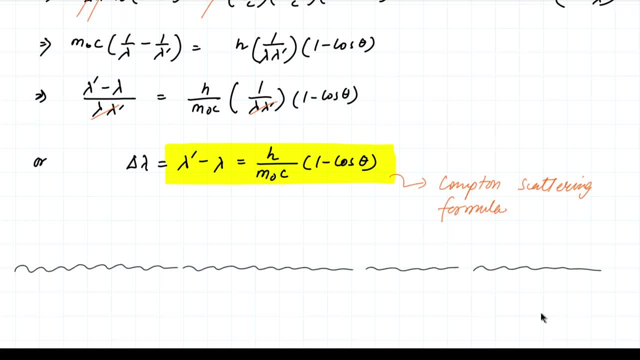 so in those interactions all the particles are relativistic, traveling at very, very high speeds and the four vector approach is very beneficial in those situations. okay, normal, ordinary moment of time or energy conservation side. it becomes very difficult to do it and even though here is the approach of quantum effect, you know an alternative approach, but the problems you will do later. 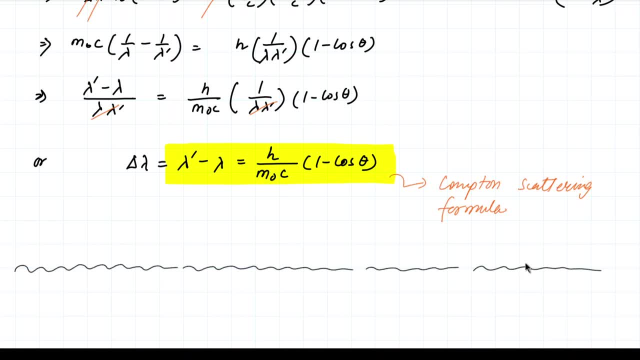 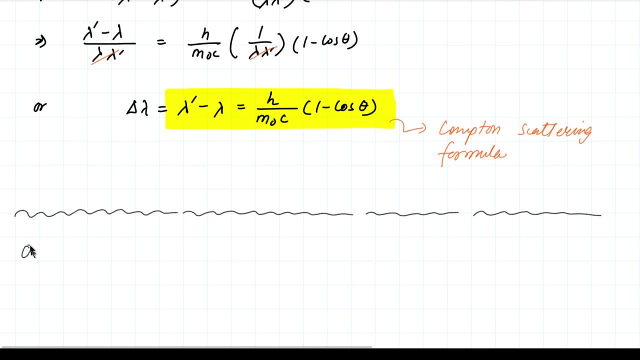 there can't be any alternative approach, so this approach is going to be helpful. so that's a little long problem that I will do in the next class. but as I want to give you a little homework, if you understand four vectors then you please try this question. and if you are able to do this problem, then maybe you know a little bit. you have become comfortable with this idea of four vectors. the question is as such: 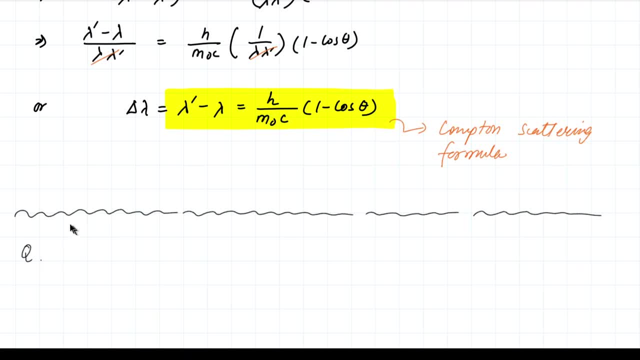 then maybe you know a little bit. you have become comfortable with this idea of four vectors. the question is, as such, as follows: can a free electron absorb a single photon? what is the answer? does anybody know? can a free electron observe a single photon? no, sir, like your score. 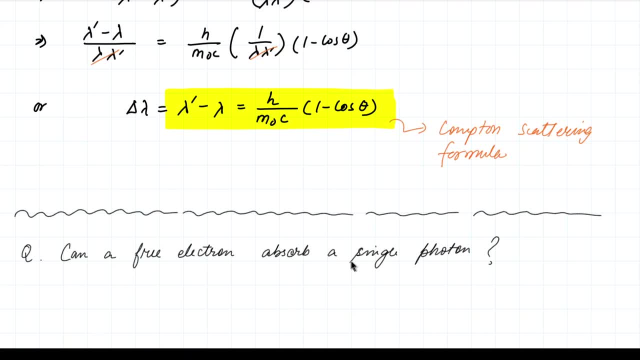 but can it absorb a single photon, completely linked atom? that would be better. you're saying the answer is no. yes, sir, answer is no. can you prove it using four vectors. let's suppose i say: can you prove it using conservation of momentum principle using four vectors? can you prove it using four vectors? 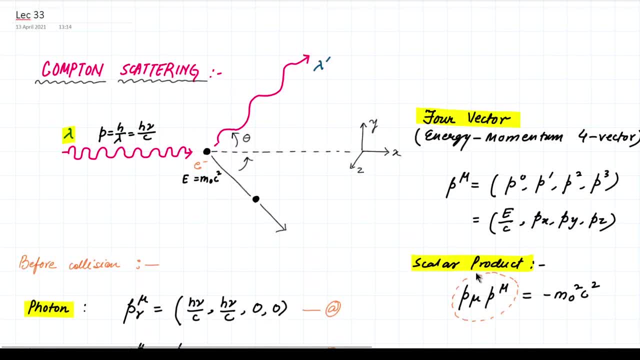 similar problem here. i took a scattered photon. you just have to remove the scattered photon and then you have to check whether the conservation of four momentum holds true or not. if the conservation of four momentum does not hold true, that means this process is not possible. that's all, did you understand? 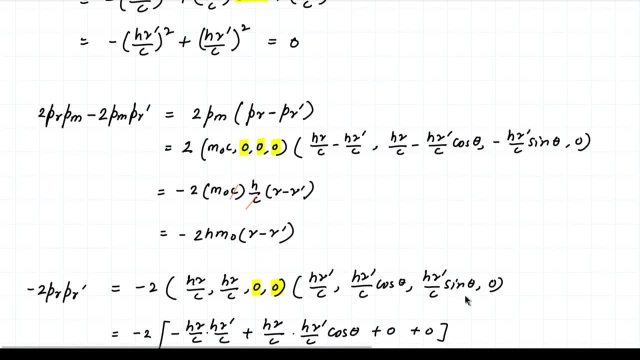 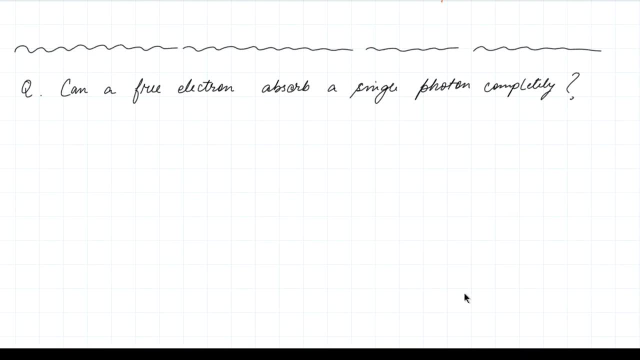 yes, sir, yes, okay, so you have to try this once at home. assume that the conservation of four momentum holds true and then try to solve it. you will find that you will run into inconsistencies, logical inconsistencies, and the reason is that this effect is not possible means if a free electron completely absorbs a single photon.